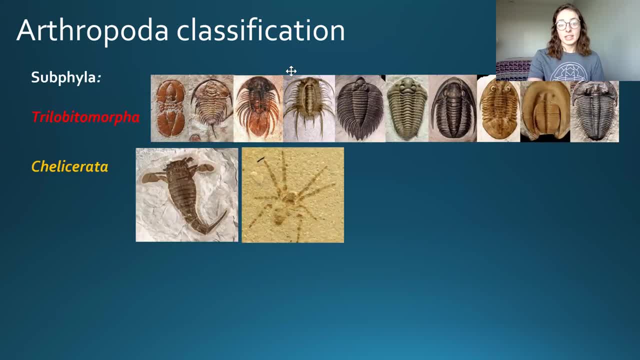 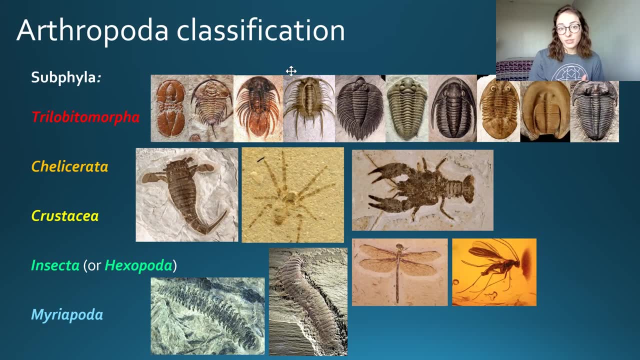 one. You have trilobitomorpha, of course, but you also have chelocerates, crustaceans, insects or hexapods And myriapods, And these last four subphyla groups we actually discussed in way more detail in the 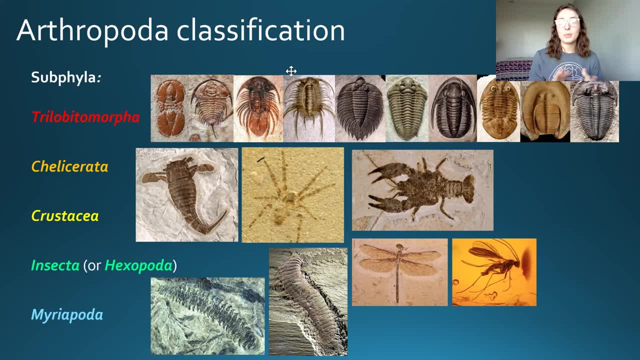 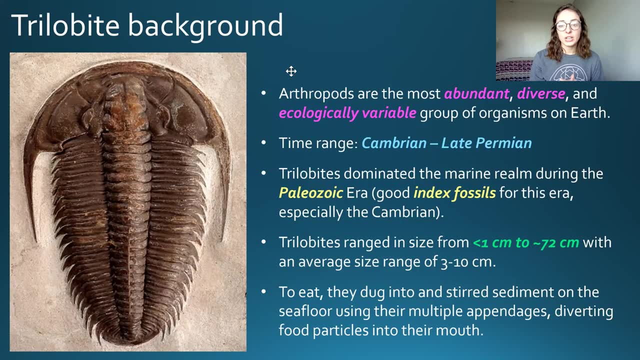 previous video after this slide, and we neglected trilobites in the last video because they're getting this video, So let's move on and talk more about trilobitomorpha. Arthropods, like I mentioned in the first video, are the most abundant, diverse and ecologically variable. 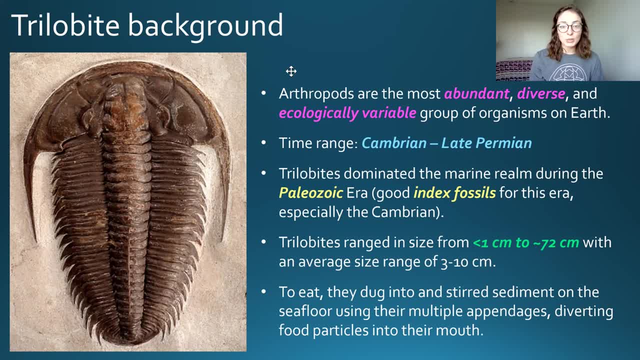 group of organisms on Earth today, as well as most times throughout Earth's history, since the Cambrian And trilobites actually aren't alive today, they're extinct. but they were really important organisms throughout the Cambrian to the late Permian or the Paleozoic era, And they 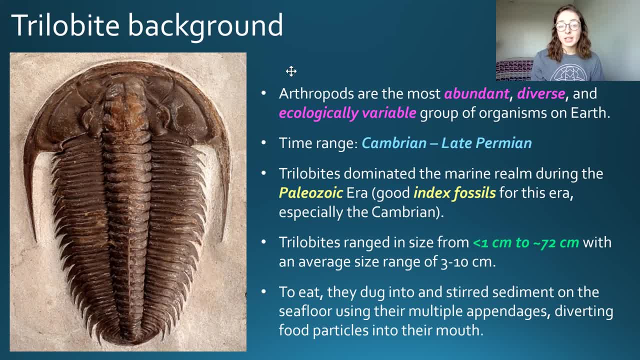 actually dominated the marine realm during much of the Paleozoic and they make good index fossils in this area because of this, especially for the Cambrian- And we'll talk more about when they dominated and when certain types dominated, and everything at the end of this video when we talk. 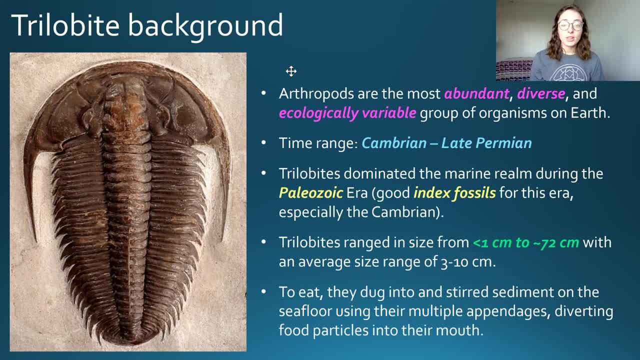 about their evolution. In terms of size, trilobites ranged from less than a centimeter to around 72 centimeters or almost a meter, But the average size of trilobites was around 72 centimeters and around 3 to 10 centimeters, so it was pretty rare that they got this big. But we'll talk later about 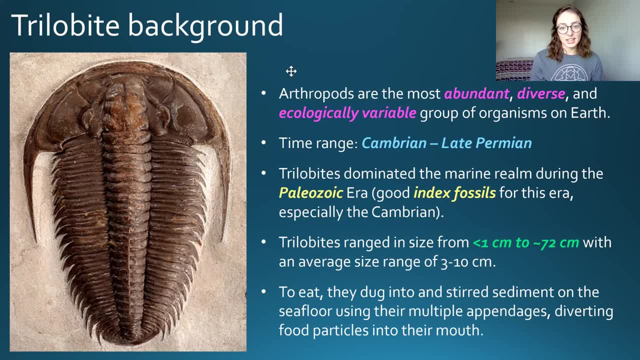 which groups of trilobites or orders of trilobites actually did get that big And in terms of ecology or what they ate. they used their multiple appendages- which is actually something we talked about in the previous video- to dig up and stir sediment on the seafloor in order to 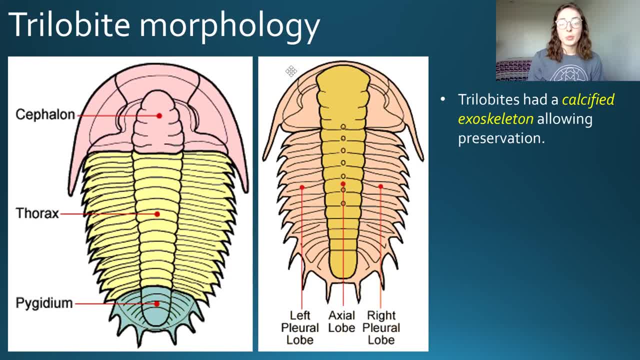 divert food particles into their mouth. But because these guys are more known to us in fossil form than actually modern form, I don't want to spend too much time on ecology or anything, because these are ancient fossils that we can only tell a lot from by studying the morphology and structure and 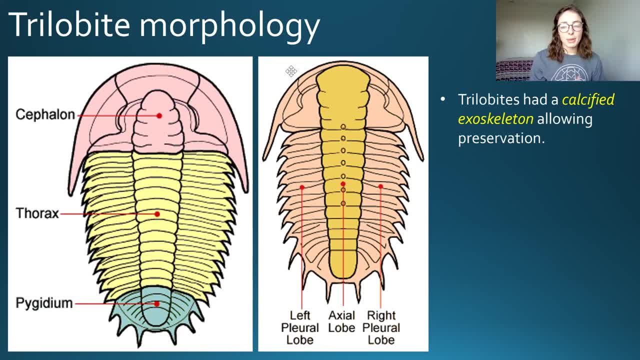 diversity of their ancient forms. So let's get into a little bit about the morphology of these ancient trilobites. Trilobites had a calcified exoskeleton, which is the main reason why they are very, very important in the fossil record of arthropods. Many arthropods just have exoskeletons. 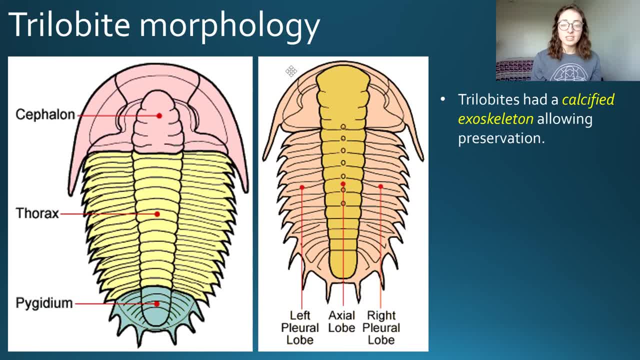 made out of organic material which doesn't preserve very well. So this calcified exoskeleton allowed for preservation And this is a very important reason why they are very, very important in the fossil record of arthropods. And the calcified carapace or body skeleton is divided. 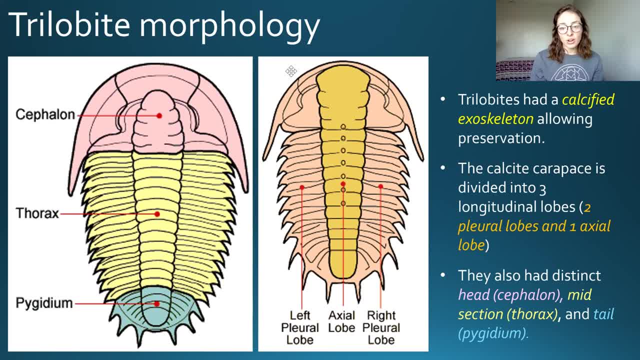 into three longitudinal sections or lobes, and these are called the pleural lobes, which are on either side of the trilobite's body. So you have the left pleural lobe and the right pleural lobe, and then you have the axial lobe, which is in the center, as we see here in this middle figure, And 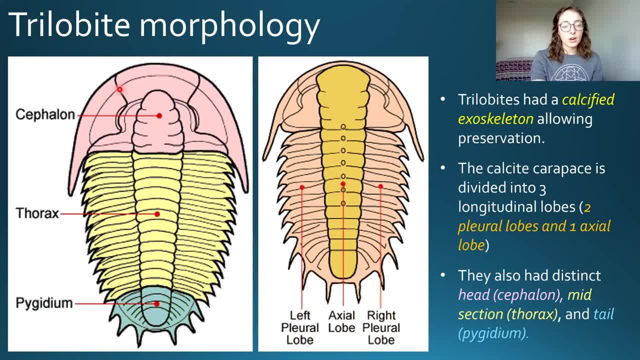 they also could be separated into three major sections, going up and down. We have the cephalon, which is the head region, We had the midsection, or the thorax, And then we had their little butt, is their pagidia, And I just think that that's a really cute name for a butt and that humans 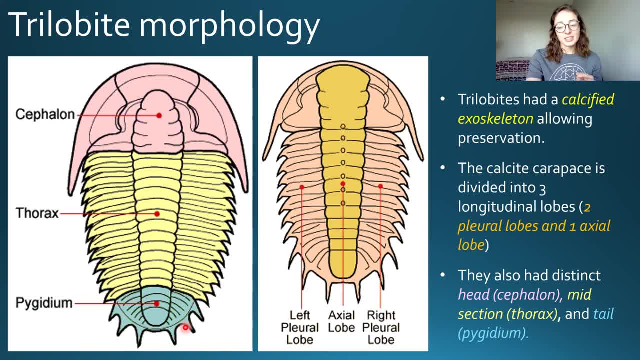 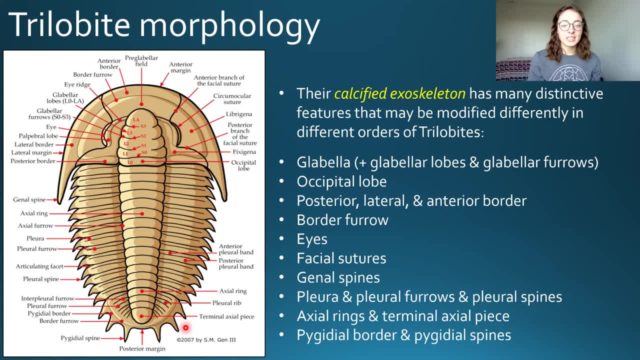 should also take up this vocabulary and call our butts pagidia, because that's just adorable. But moving on, there's a lot of other distinctive features that might be modified in different orders of trilobites, which is why it's important to understand where they are located on the 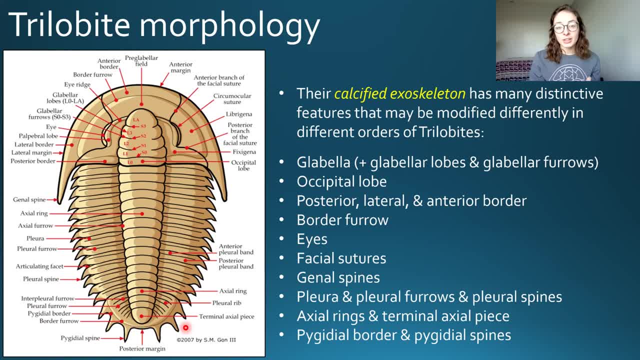 trilobite and how they might take their form, And so we're going to label those now in this figure. First we have the glabella, which I like to call the nose of the trilobite, even though it's not. 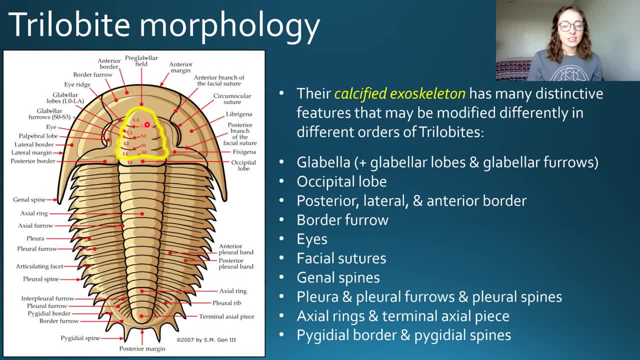 it's the glabella. I just think it looks like a little cute nose on their little cephalon. But anyway, this glabella can have glabellar lobes and glabellar furrows which separate the lobes on the glabella And the lobes and furrows, as well as the glabella itself can change in shape. 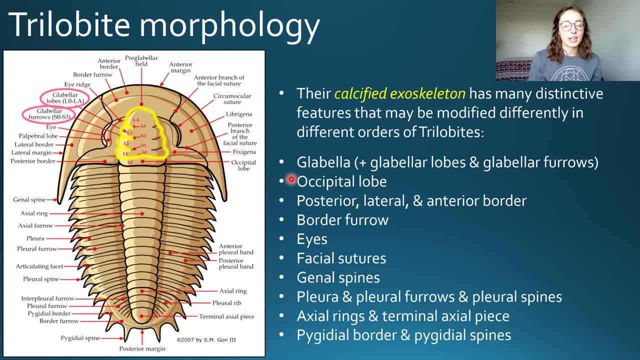 and structure, depending on what order of trilobites you're looking at. For example, the glabella sometimes has this triangular shape in which it tapers or narrows toward the anterior of the cephalon, And also some trilobites will just call that glabella, a tapering anteriorly glabella. 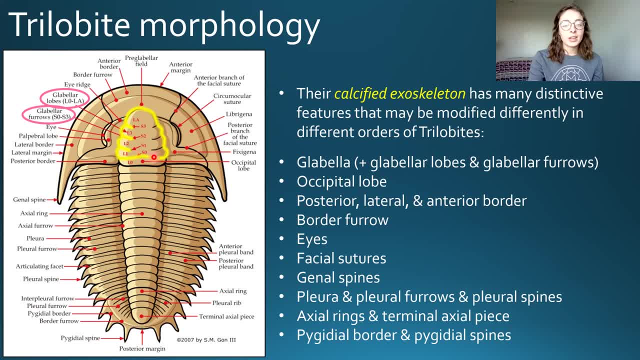 whereas some groups of trilobites have an extending anteriorly glabella, in which case it would be widening toward that anterior edge of the cephalon rather than narrowing. The next distinctive feature is the occipital lobe, which is right below the glabella, And then you also have the 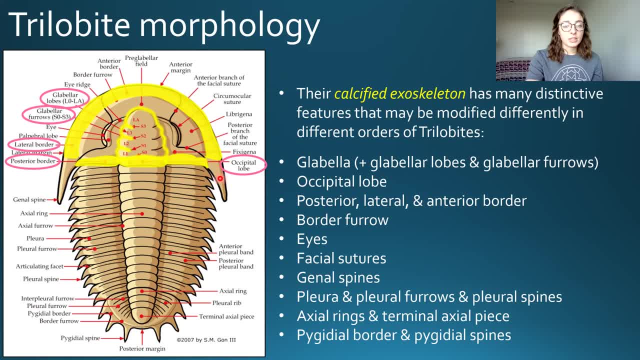 posterior border. on either side of that lobe You have the lateral border, which is the border along the cephalon, along the lateral sides, And then you have the anterior side of the glabella, which is the the anterior border, which is the part of the border that is on the anterior end of that. 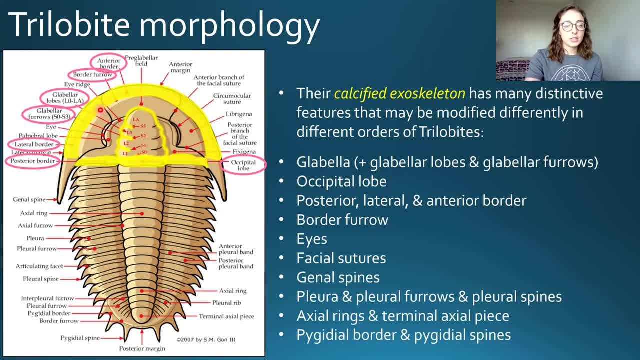 cephalon. You also have the border furrow, which is the line or periferation that kind of separates that border with the rest of the cephalon. Additionally, you have eyes on trilobites. They actually have really sophisticated eyes we'll talk about in a couple slides And these are shown. 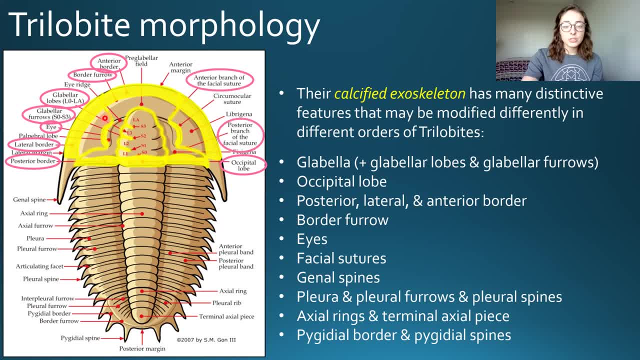 to be these little crescent-shaped things right here. They also have facial sutures, which are pretty important- and we'll talk about those on their own slide as well, And these are shown here in this highlighted line, and they can take different shape depending on the type of trilobite. 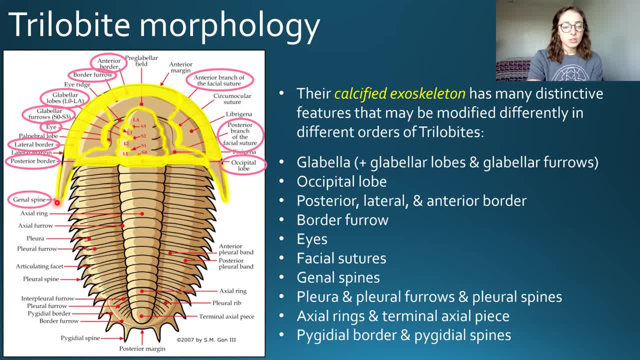 you're looking at again. Additionally, you have genital spines which are shown coming off the sides of the cephalon and down toward its thorax, And these spines can sometimes be completely absent in certain groups of trilobites, or sometimes they're very long and protruding in. 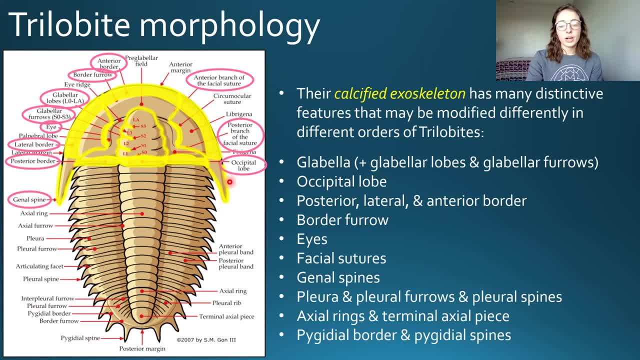 other groups. So these are also a distinctive feature that are good to look for. And then, in terms of the thorax, you have the thorax, which is the thorax, that's the most common type of trilobite. And then you have the thorax, that's the most common type of trilobite, which is the 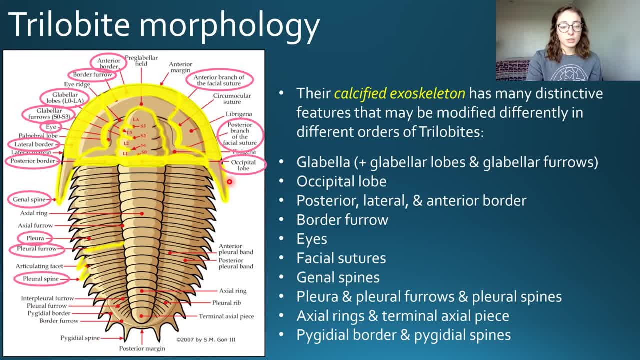 thorax. We have the pleura and pleural furrows, as well as pleural spines as well, And the pleura is just each one of these little segments. You have the furrow in the middle of the segment and the spines coming off the sides again and again. Sometimes you don't have these spines. 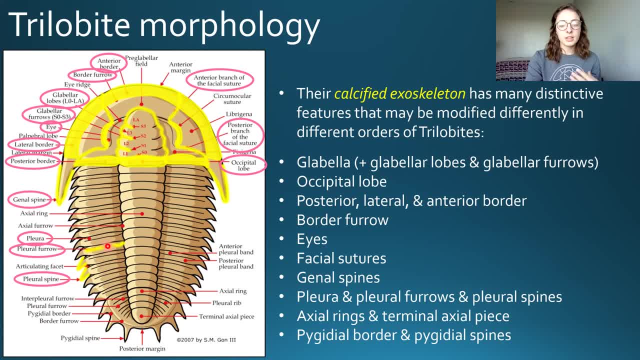 on the pleura, and sometimes you do, depending on the group of trilobites. Also, there's axial rings, which are the rings that are on the axial lobe or center part of the trilobite, And these are segmented rings that can be numerous and they can also be very large, And these are 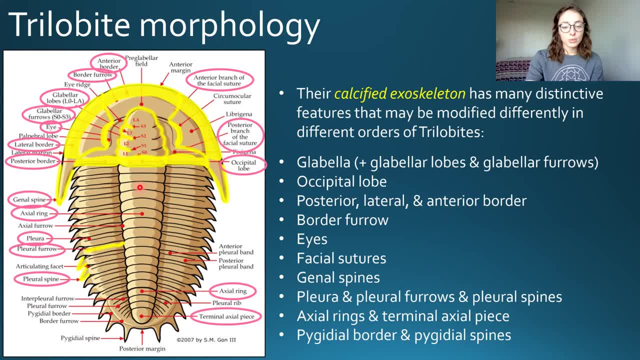 very few, depending on the trilobite order again. And then there's the terminal axial piece, which is the last axial piece of that axial lobe on the trilobite. Then you also have the pagidial border, which is the same as the cephalon border that we highlighted up here. It also has a 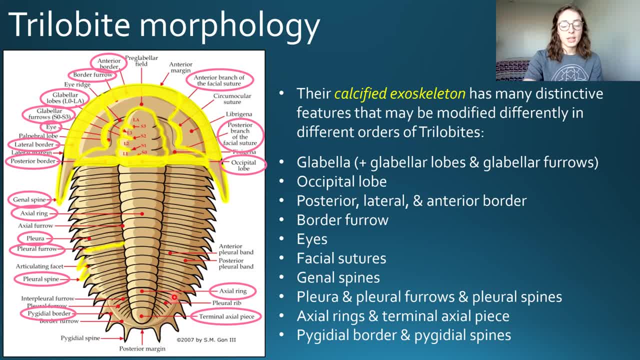 border furrow, but instead of being on the cephalon, it is on the pagidium, And then you also have the pagidial spines, which can be present and cannot be present, depending on the trilobite group again. And these spines can also, if they're present, be short or very long, And 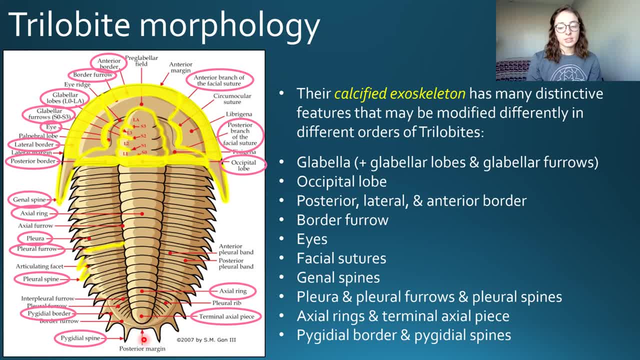 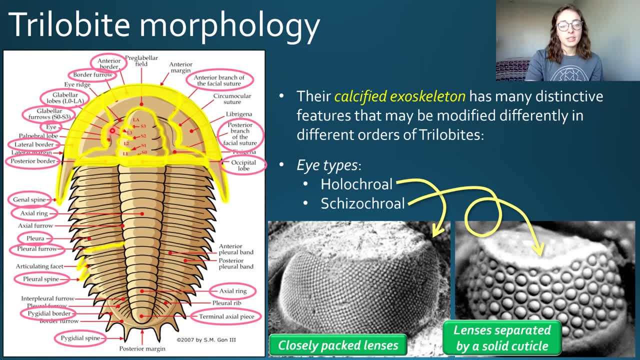 then you can also have one right in the middle in certain groups of trilobites, And so we'll show examples of that later. So let's move on and talk a little bit about these eyes. that can be different, So we labeled the eyes in the trilobite. They're right here, these crescent-shaped little. 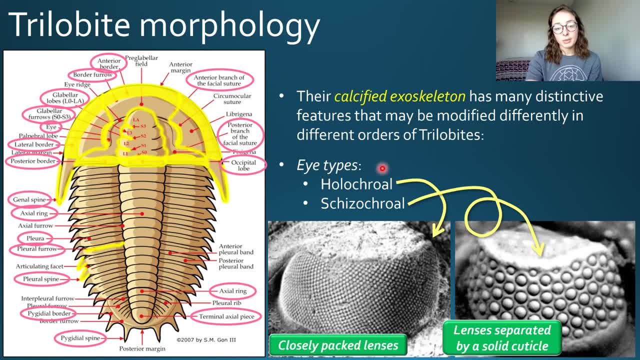 things, And these eyes on the trilobite are typically one of two types. These are holochral and schizochral eyes, And holochral eyes are shown here in this left picture. These are very closely packed lenses. And then you have schizochral eyes that actually are lenses separated by a solid 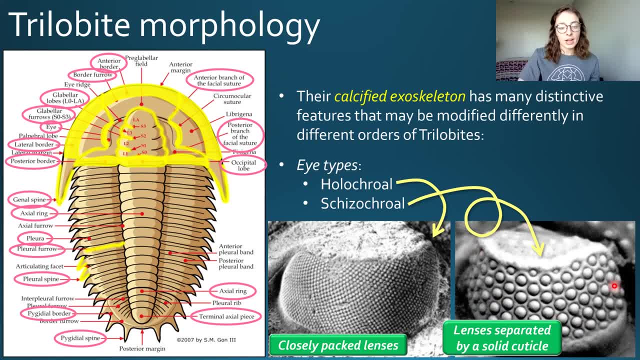 cuticle, which are the more sophisticated type of eye for trilobites and can be seen in some of the orders. But actually many trilobites evolved to lose their eyes and become blind because where they were eating and what they were digging up and everything and how they were doing it was. 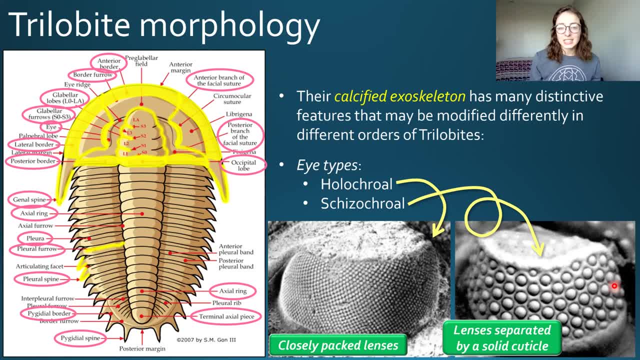 actually in the dark on the seafloor And so they just really didn't need their eyes. So a lot of them evolved in the way of losing their eyes and becoming blind, and that was actually beneficial for them. But still some of them actually evolved more complex eyes like these skylight eyes. 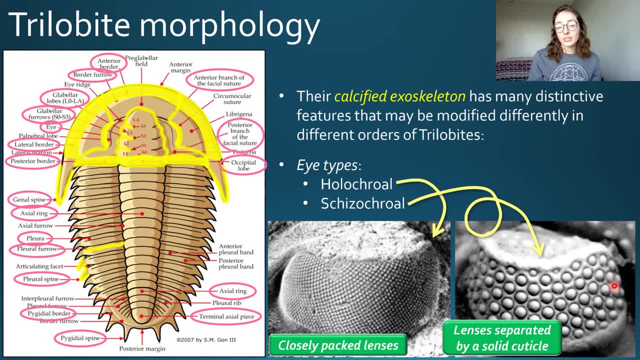 holochral eyes just depending on where and how they lived and if they needed them and if it was a beneficial trait for them to keep. So the eyes of trilobites can be a pretty distinctive feature, because sometimes you might be looking at an order and you're like: this one has eyes. this one did. 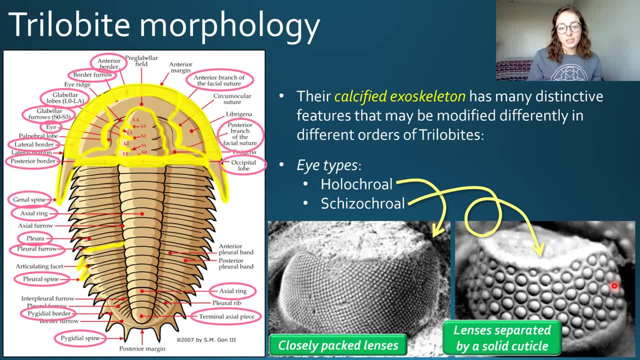 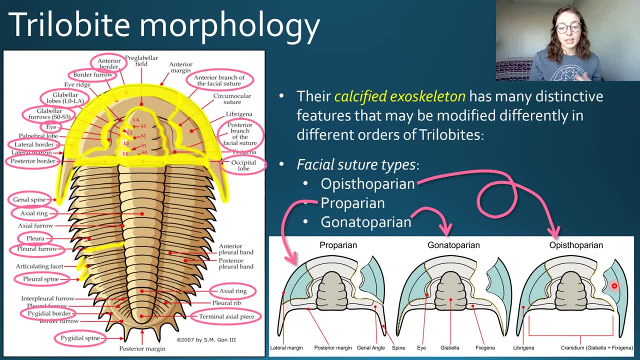 not have any eyes, So sometimes that can help when identifying what trilobite you're looking at in a fossil. Also, trilobites have facial sutures, which I mentioned earlier, And these can be one of three main suture types typically, And these suture types include properion, gonatoperion and 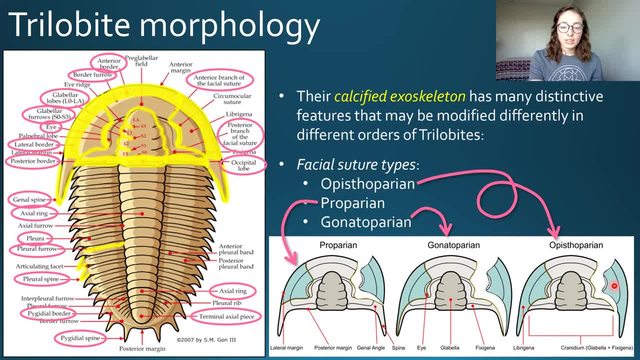 epistoperion, And these suture types are shown here At the bottom right. what we have here is properion, where the suture emerges in front of the genital angle, which is the angle here at the edge of the cephalon, Whereas gonatoperion actually 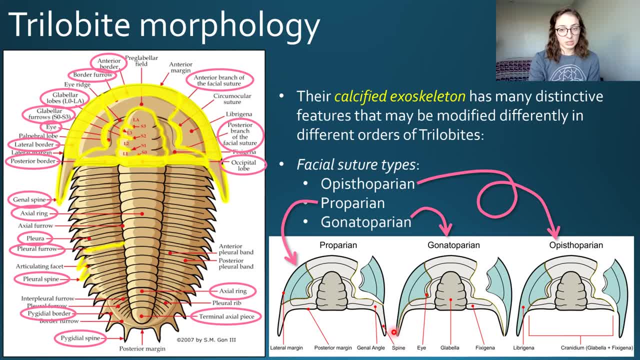 splits the genital angle and goes down the genital spine. if there is a genital spine present And epistoperion actually cuts out behind the genital angle, And that is actually what we see in the example in the left figure- We see that that facial suture actually cuts out behind the genital angle. 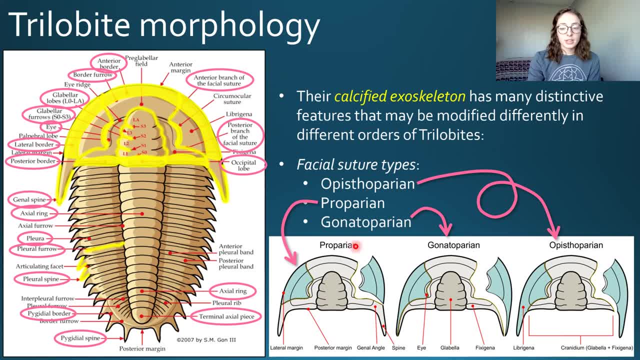 and includes the genital spine and everything. So that is epistoperion, And then you have gonatoperion and properion, And these can be distinctive features in certain orders of trilobites as well, And so we'll point out as we go through the classification in different groups of trilobites. 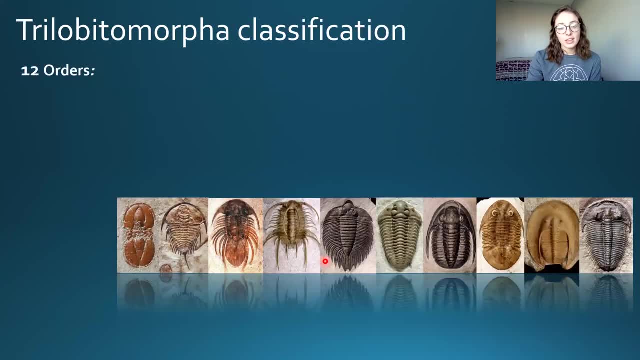 later which ones have which facial sutures. So let's get into the 12 different orders of trilobites, because this is, I'm sure, what everybody's been waiting for. If you are in any invert paleontology class, you likely have a professor that loves to quiz you on these 12. 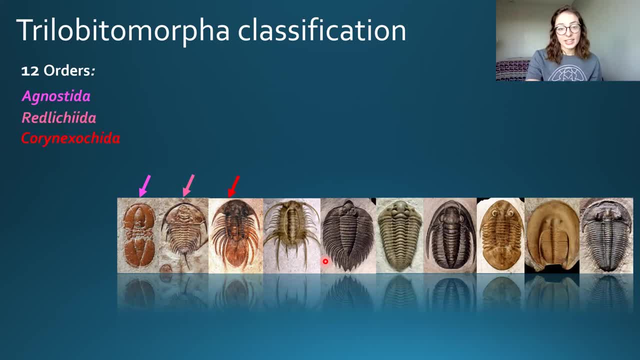 orders of trilobites. These include agnostida red lichida corinexikida. I hope I'm saying that right, ticoparida? sorry, these aren't in order. that's the one over on the. 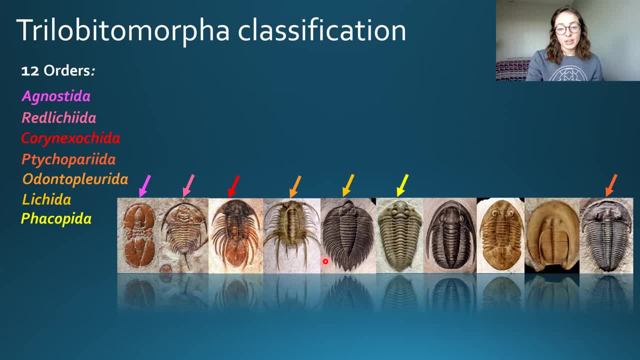 right odontoplorida, the one with all the spines, lichida phacopida proetida, asafida trinucleata, which is sometimes clumped in with asafida. so we're just putting the arrow in the same place. 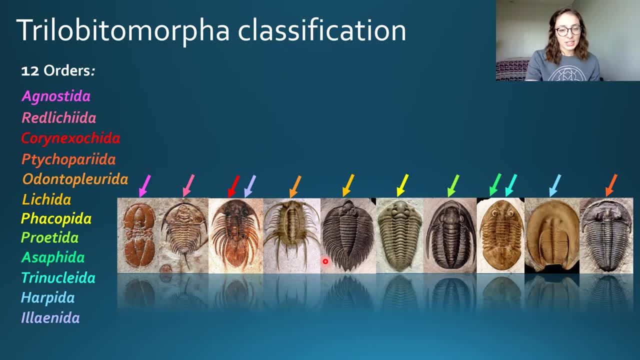 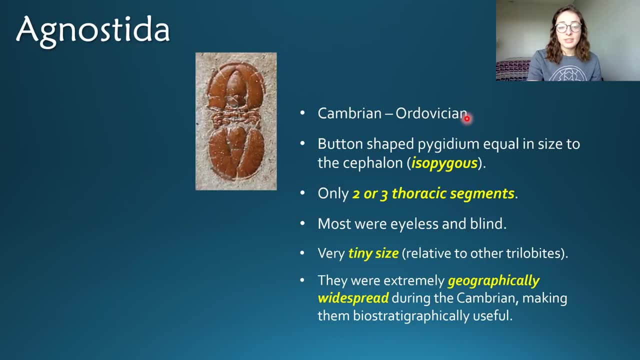 basically harpida and the alanins, which are also sometimes clumped in with the corinexikids. So let's go through these and their features one by one. First we have agnostida, Agnostids, lived shaped pygidiums which are so dang cute and the similar size of their pygidium to their cephalon. 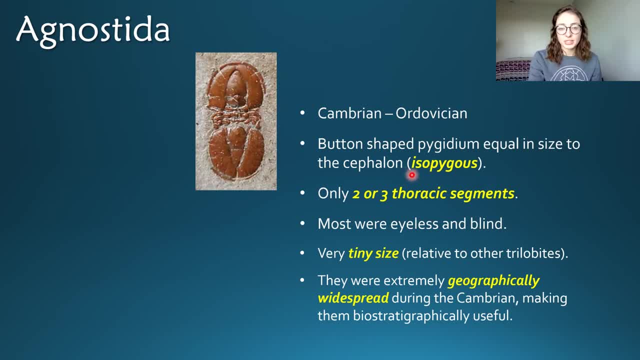 makes them fall under a category called isopygis, which just means the same pygidium size as their cephalon size. And then they also have only two to three thoracic segments, which makes them pretty distinctive, because a lot of the orders, as we'll see later, have a lot of thoracic segments, like 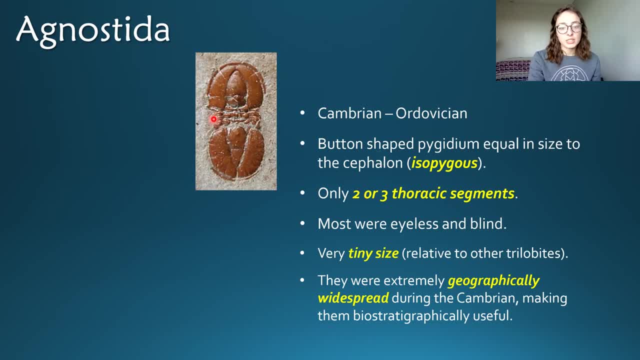 up to 10, which is a lot more than two or three. so sometimes if you only see two or three thoracic segments, you can right away pretty much say that's an agnostid. Another distinctive feature of them were eyeless and blind, and so if you don't see any eyes on the cephalon, then that's. 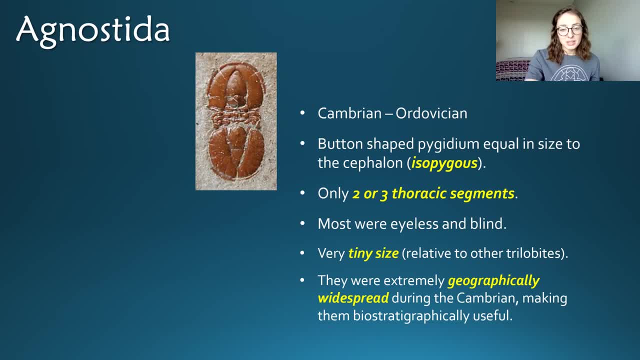 another reason to think that this might be an agnostid. Additionally, most of them were very tiny in size relative to other trilobites, and so looking at their size, or if you have another trilobite in the rock you're looking at and you can see that these are very small, then that's. 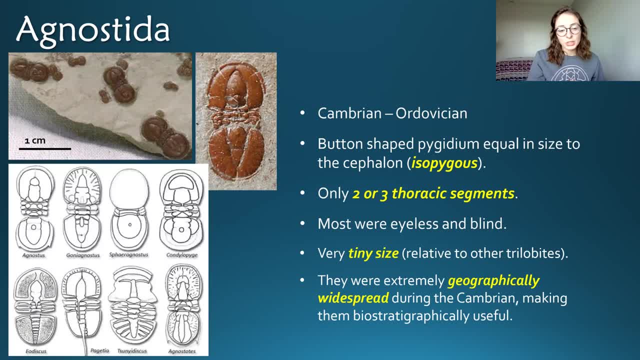 another reason to think. maybe they're agnostids And just for reference, here's some more pictures of their morphological diversity and different genera that are included within agnostida. We have the agnostis, goniagnostis, spheroagnostis and the agnostida, And then we have the agnostida. 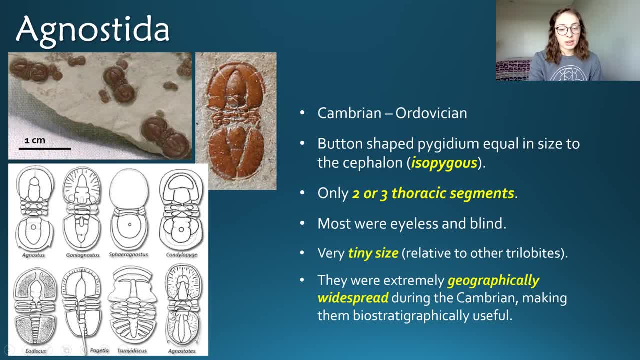 and more, and these all have isopygous bodies with a pgidium that is button-shaped and roughly equal in size to their cephalon. Most of them don't have a posterior spine, but this group, the pagetia, does, and so maybe that would be a distinctive feature. if you see the isopygous. 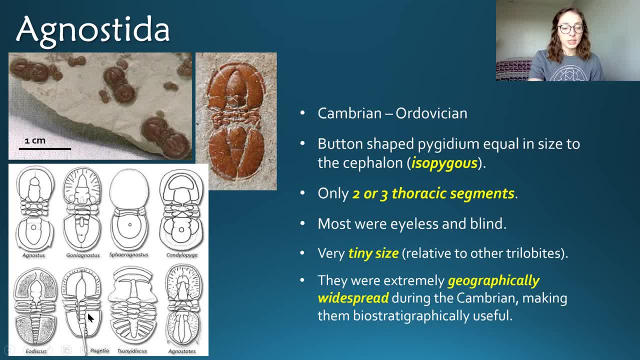 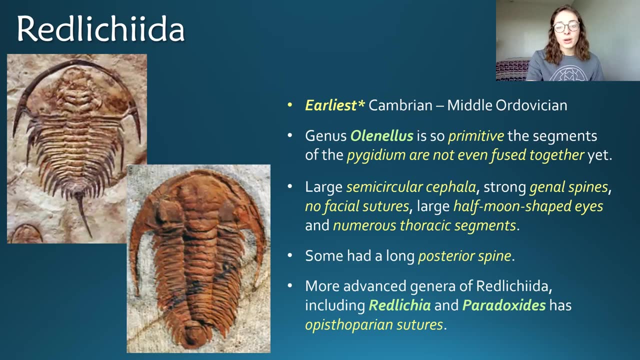 small size of the trilobite and then a posterior spine. And the last thing I want to mention about these guys is that they were extremely geographically widespread during the Cambrian, and that makes them really useful for biostrategic. Moving on to red lichida: red lichids went from the Cambrian to the middle Ordovician. 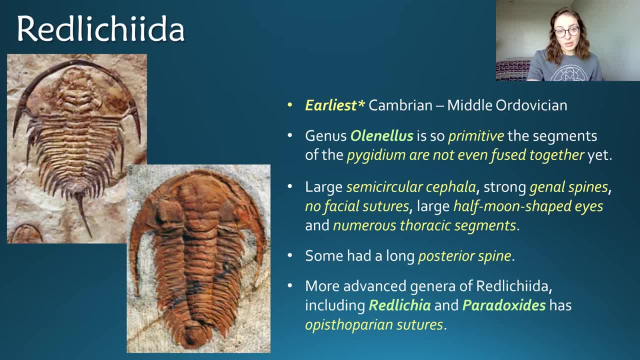 but they were actually the earliest evolved trilobites, or at least from what we know from the fossil record we have, And the genus Olenellis is thought to be the most primitive form of trilobites that led to the evolution of all the other trilobite groups And one of the features 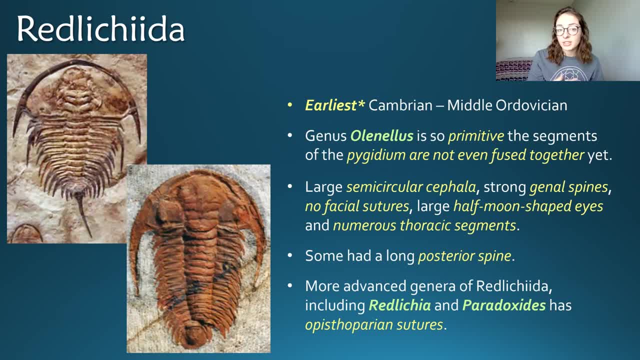 that makes this Olenellis genus so primitive is that the segments of its pgidium aren't even fused together yet, which is a common characteristic of all other trilobites. Additionally, red lichids have a large semicircle cephala, as we can see in these pictures, Their cephala. 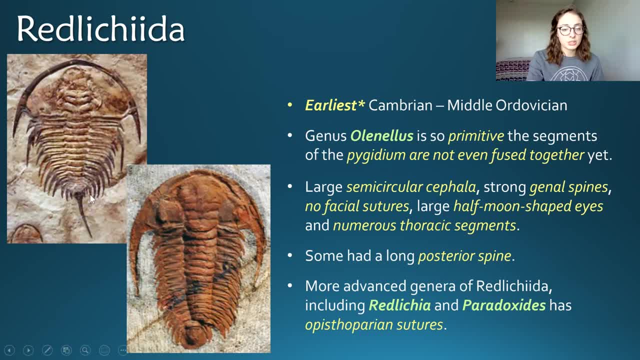 which is just plural for cephalon, is pretty big compared to, especially their pgidium, and so they're definitely not isopygous. They have a much larger cephalon than their pgidium and even their thorax, And they also had strong gentle spines, as we can see coming off their 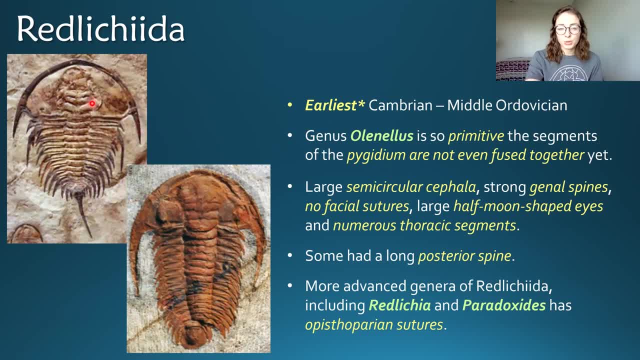 cephalon And they had no facial sutures, which is probably another primitive characteristic of these guys. Additionally, they had numerous thoracic segments. We can see they had a lot more thoracic segments than agonists And they have half moon-shaped eyes. Some also had a posterior spine, as we can see. 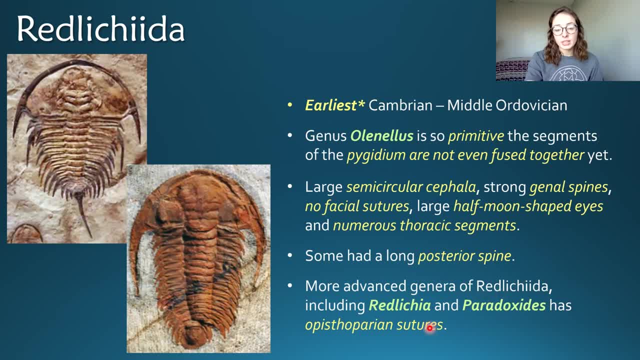 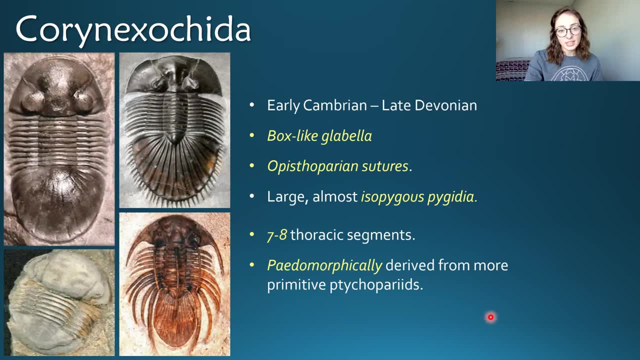 in the top left figure And more advanced genera of red lichids, including red lichia and Paradoxides, had evolved opisthoperian facial sutures. Next we have the Corynexicans, which went from the early Cambrian to late Devonian and had a box-like glabella such 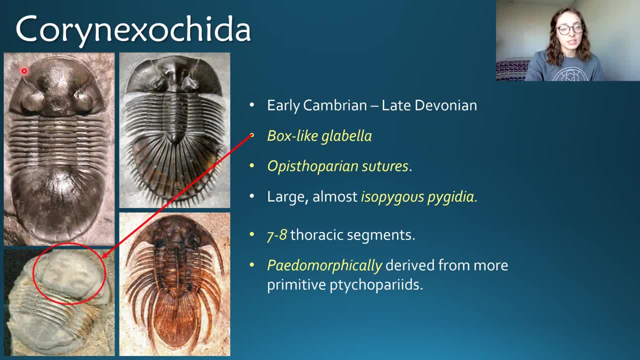 as shown here, But they also sometimes had anteriorly extending glabellas, as we see in this guy up here. This is another example of what we call the PDRN, which is different from the one we labeled. So there's an example of one that widens toward the anterior of the cephalon rather than narrowing. 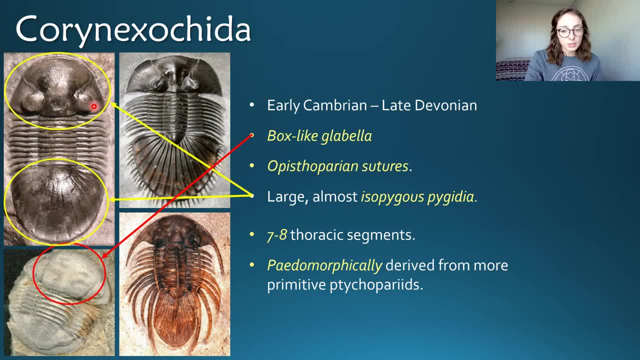 And they also had opisthoperian facial sutures similar to the more evolved red lichids that we just talked about. They also had large isopygous pgidia. These pgidia were similar in size, if not greater in size than the cephalon, making most of them isopygous, And they had seven to eight. 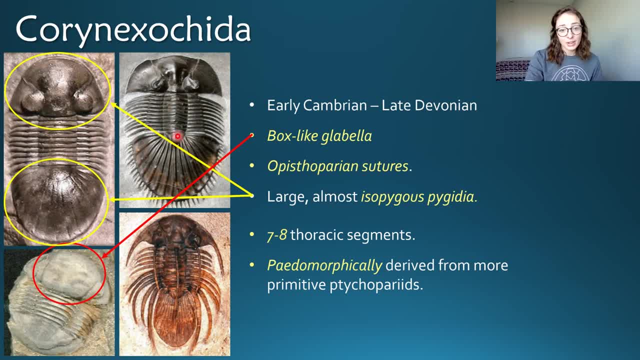 thoracic segments which, if you feel like counting the thoracic segments when identifying the corynexicids and many of the features listed here, are thought to have panamorphically derived from more primitive Tychoparidae, which is the 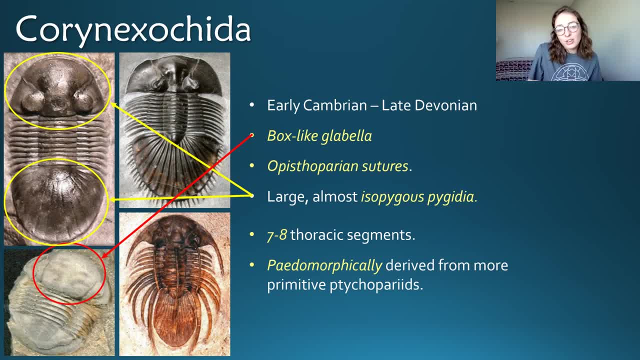 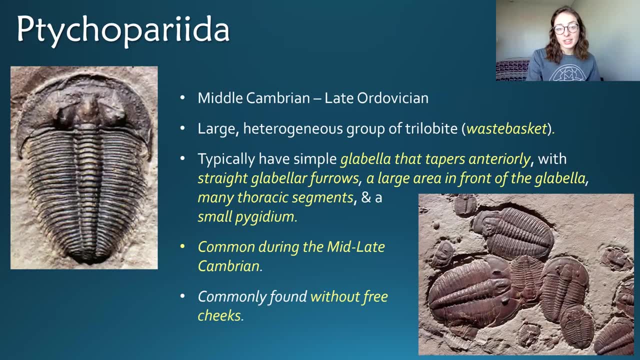 order we'll talk about on the next slide, But basically this means that many later evolved corynexicids might have derived some more juvenile features from the Tychoparidae group, which is the Tychoparidae as we can see. that went. 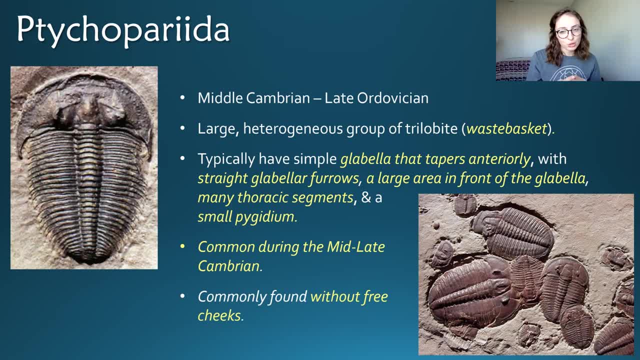 from the Middle Cambrian to the Late Ordovician. These were a large, heterogeneous group of trilobites, often thought of as a wastebasket because of how many different trilobites are put into this group, but basically these typically have a simple glabella that tapers anteriorly, so we can see that. 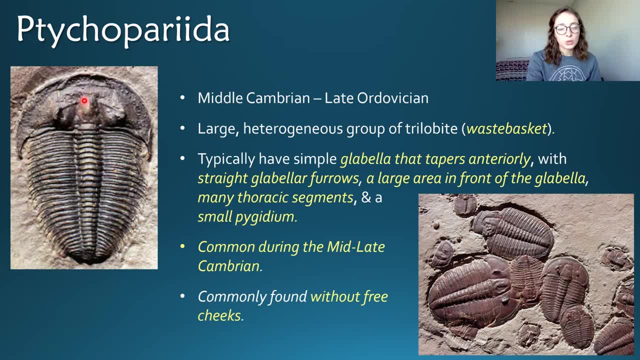 this glabella here has a more triangle shape that tapers toward the anterior of the cephalon or narrows toward it, similar to the trilobite on my shirt. Maybe this is a Tychoparidae And it has straight glabella furrows, so the furrow. 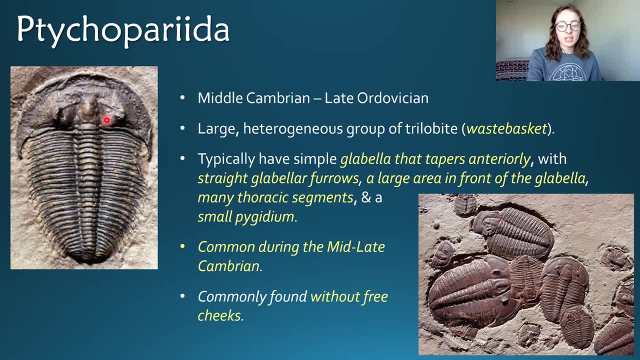 at the base of this glabella is straight rather than curvy. Also, it has a large area in front of the glabella before you reach the border, and many trilobite orders actually have glabelas that go in the middle of the glabella, So this is a very common type of glabella. 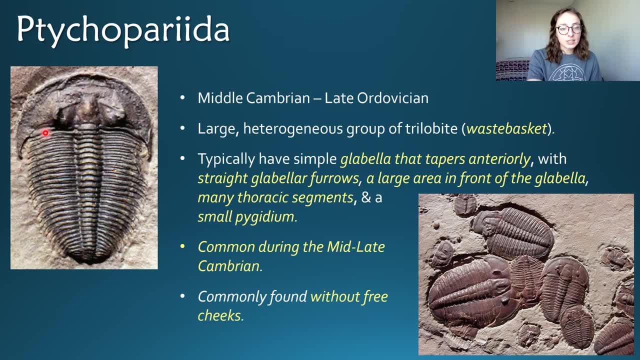 Straight out to the end of the anterior of the cephalon, whereas Tychoparidae actually has this big space. Also, they have many thoracic segments, as you can see here on its thorax, as well as the picture to the bottom right, as well as 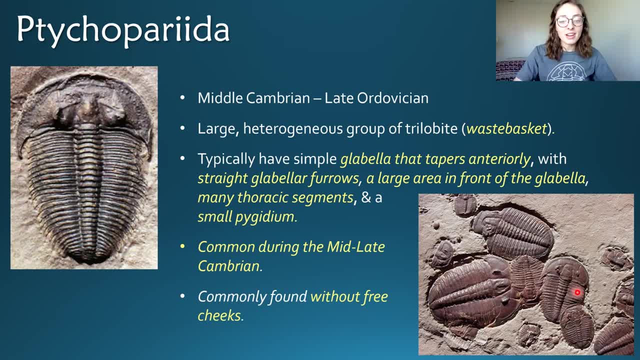 my shirt here- Many thoracic segments on Tychoparids. Also, they have a little tiny pagidium which is at the bottom here, and this is another distinctive feature of Tychoparids. Also, this group was common during the Mid to Late. 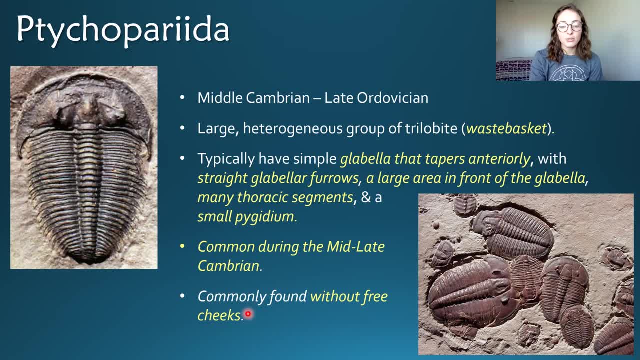 Cambrian, and they commonly are found in the fossil record without free cheeks. The free cheeks of the trilobite are basically the parts of the cephalon that are outside of the facial sutures, Because the facial sutures are kind of 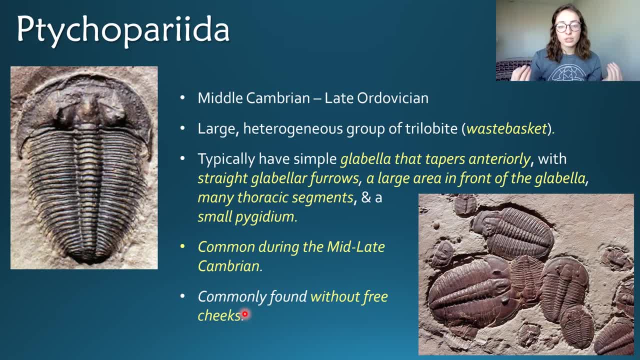 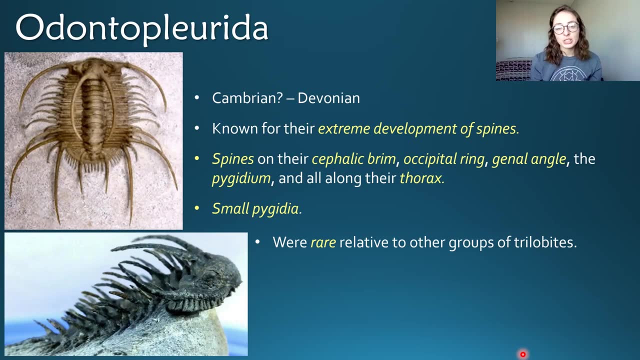 like peripherations. sometimes the free cheeks can break off during burial and preservation, making them be preserved without these cheek parts, as we can see in the figure to the bottom right. Next we have Adontoplurids, which went from the Cambrian question mark to the Devonian and there's just a question mark here. 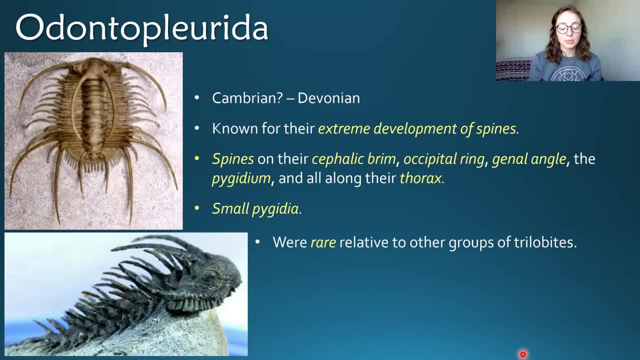 because it's really uncertain exactly when they evolved in the Cambrian, or maybe if they evolved in the Cambrian, or if they evolved in the Cambrian, or maybe if it was Ordovician. So that's still up for debate. but basically these 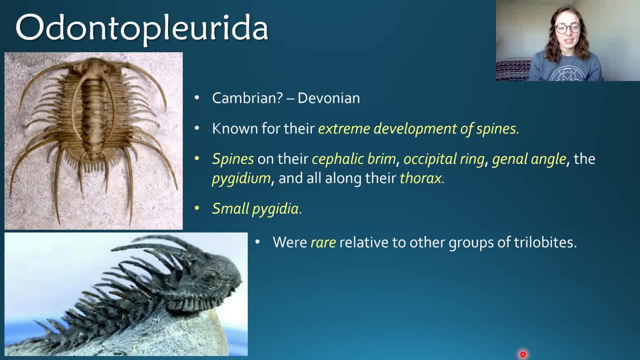 are one of the more distinctive orders of trilobites. in my opinion, probably one of my favorites, because they have so many crazy spines And obviously these spines are sometimes really hard to actually become preserved, perfectly like in these specimens we have here. So it's hard to see these guys in the fossil. 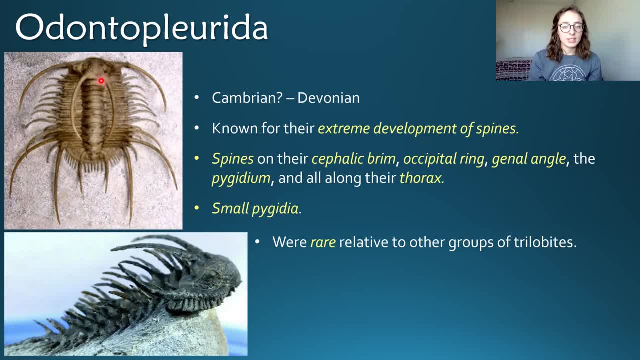 record that, often with all of their ornaments and therefore sometimes hard to find Adontoplurids and identify them correctly. But basically their distinctive features include spines on their cephalic brain, as we can see coming out here. They also have spines on their occipital ring. 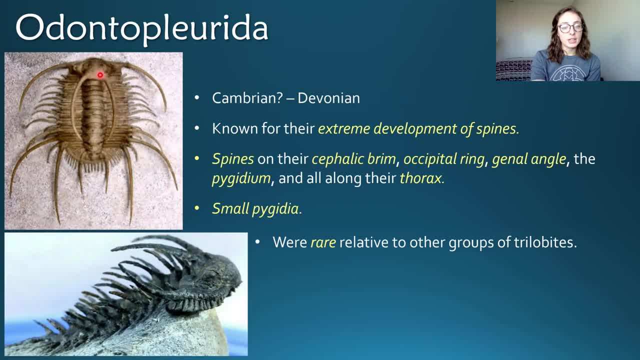 shown here. This is the occipital ring, like below the glabella, and this has spines coming off, going out of the picture toward you and toward their back or posterior region of their body, And then they have spines at their general. 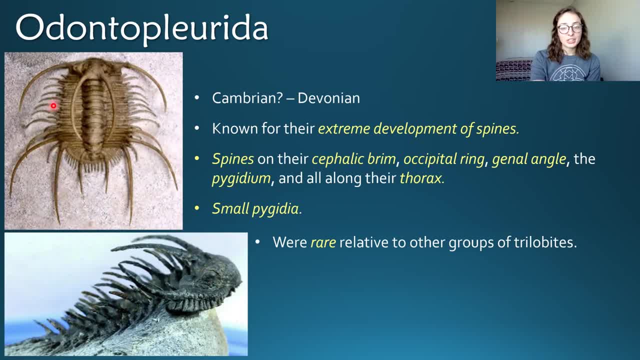 angles, spines on their pagidium, spines all along their thorax, and then they have a small pagidium, And these were actually rare relative to the other groups of trilobites during their time range and therefore I don't know if you've heard of them. 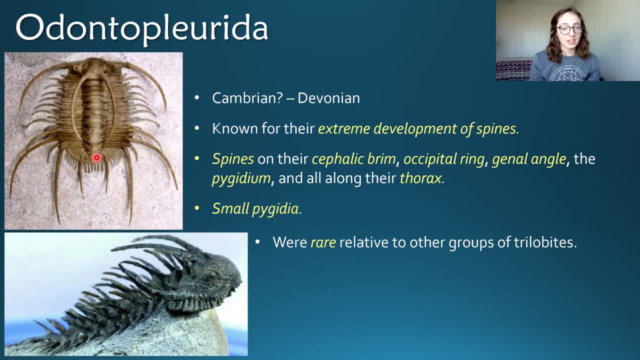 Not only are they rare in the fossil record just due to the fact that they weren't as common as the other trilobites in life, but also due to the fact that sometimes their spines get broken off and then their segments get broken off because of that, and their fossil record is kind of more. 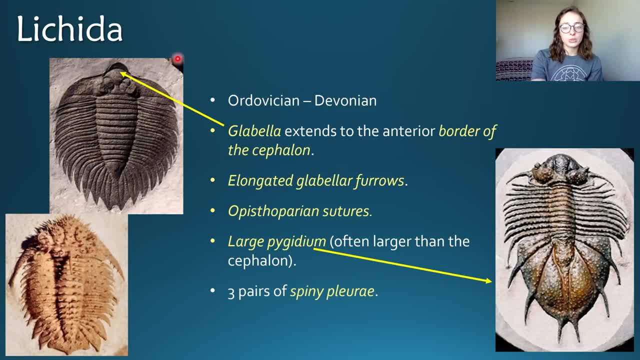 sparse. Next we have the Lichids, which went from the Ordovician to Devonian, and they have a glabella that extends to the anterior border of their cephalon. So instead of having a space there, like the Tychoperids did, as we saw, these actually have a glabella that. 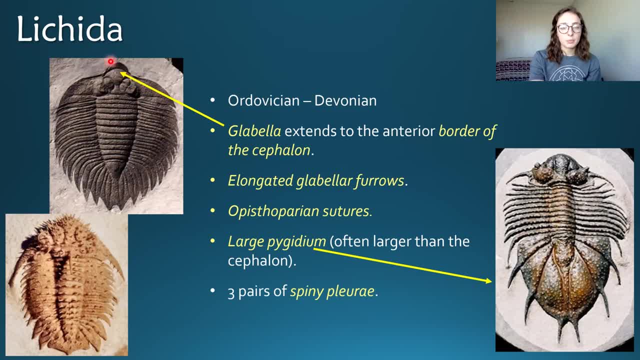 goes right out to the end and even kind of protrudes past what would be the cephalic brim. And then they also have elongated glabellar furrows, epistoparion facial sutures and a large pagidium, as we can see in this figure to the right, sometimes even larger than their 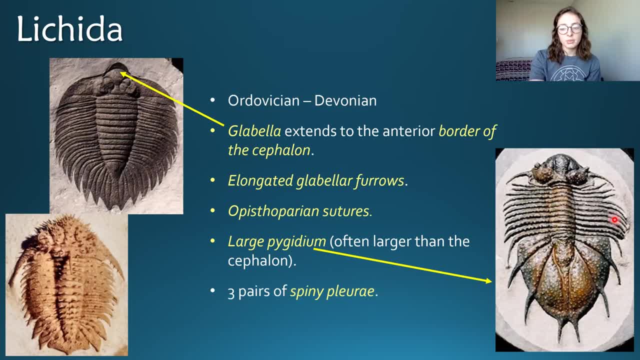 cephalon. And lastly, they also often have spiny pleurae, which can be seen in the pleurae of this guy to the right with the big pagidium, And then you also have spiny pleurae over here on this. 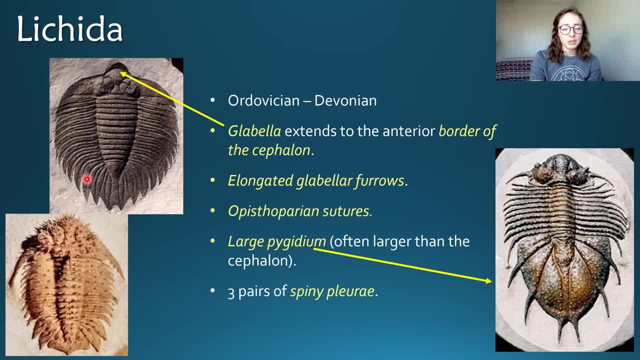 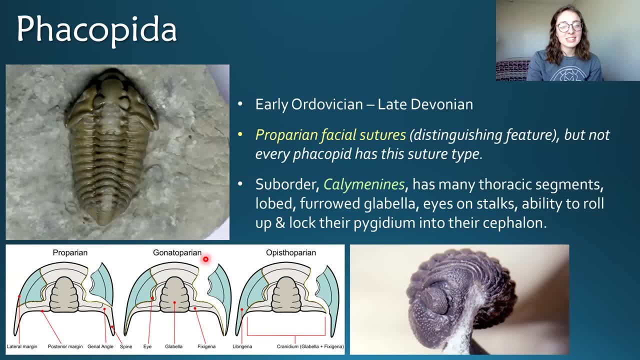 ornamented dude at the bottom and then spiny pleurae that kind of goes right out to the end, which kind of look more like feathery pleurae on this guy at the top, but these are actually pleural spines, not feathers. And next we have Phacopids. I want to spend a little bit more time. 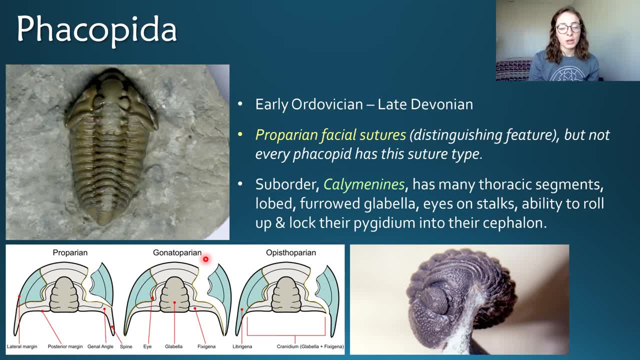 on Phacopids because they have some really distinctive groups that we're going to talk about. So basically, Phacopids went from the early Ordovician to late Devonian and this obviously isn't a long time range, but actually the fact that they have a short time range makes them 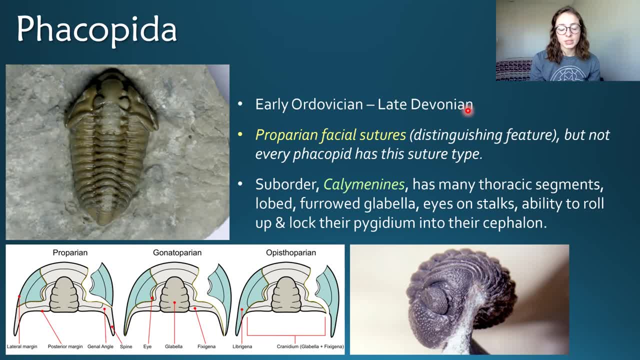 better index fossils. So this is actually a pretty nice time range to see with something that was so geographically widespread and distinctive in the fossil record. Also, these guys have Proparian facial sutures, which is their distinguishing feature because, as we've talked about in the previous Orders, you've seen that many of them have either. 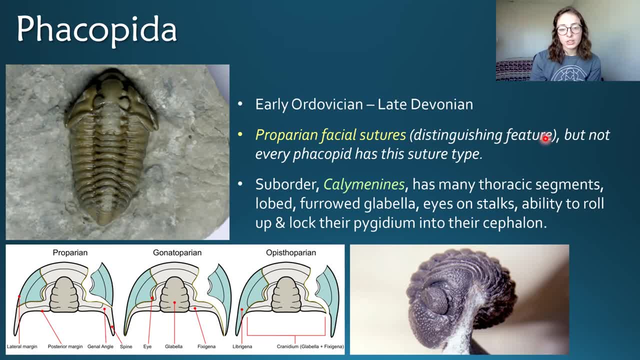 no facial sutures or Epistoparian sutures, whereas Phacopids are the only group today known to have Proparian facial sutures. However, not every single Phacopid has this suture type. It's just a distinctive suture type for this Order. So if you see Proparian facial sutures, you know you're. 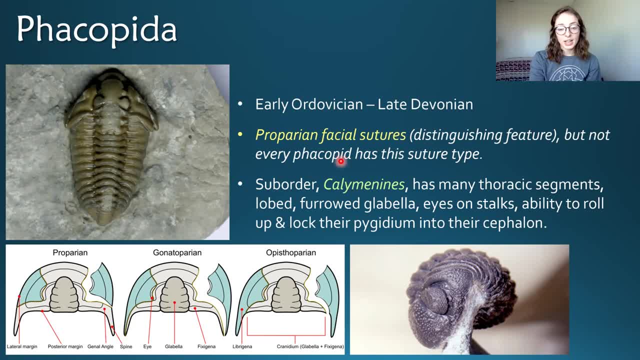 within the Phacopid group. Also, they have a sub-order group called Calaminines, which is actually shown here to the picture on the left. So if you're looking for a little bit more detail, not the bottom picture- so that is not a Calaminines Phacopid, It's a different kind of 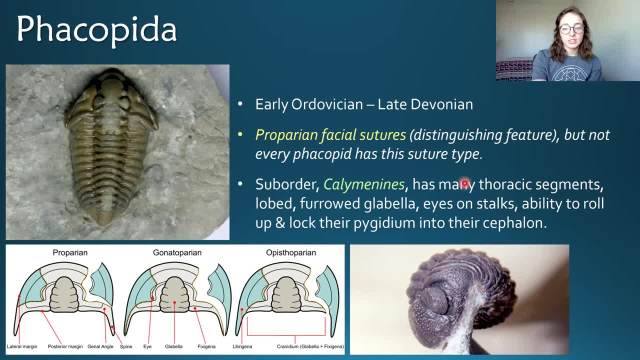 Phacopid we'll talk about later, But basically, if we look at the figure to the left, you can see that these have many thoracic segments lobed and furrowed. glabella as we can see with the lobes. 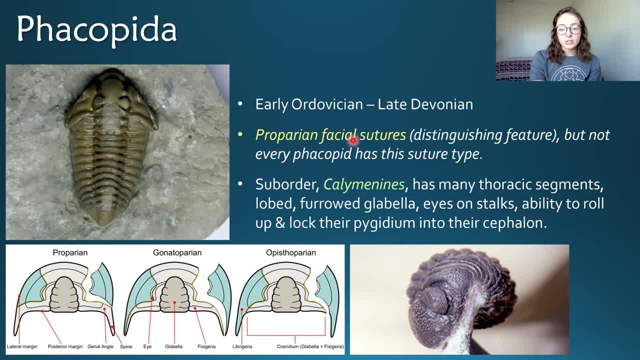 and the furrows on the glabella of this little dude. Also, they have eyes on stalks, so you can kind of see one of the eyes protruding here, but it's hard to see. Basically, take my word for it. 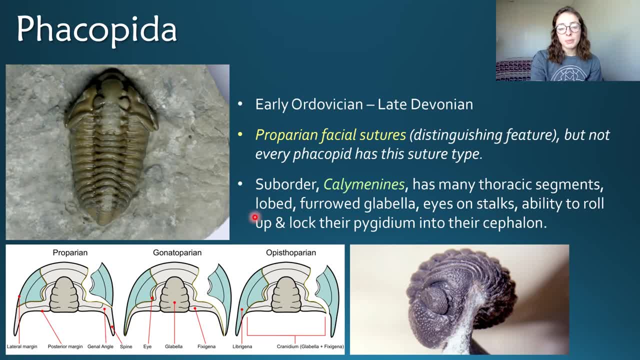 they had eyes on stalks. And then they also have the ability to roll up and actually lock their vaginium into their cephalon and stay rolled, kind of like that. It's kind of like how a roly-poly rolls up, but instead of just rolling, they actually lock themselves into place in that. 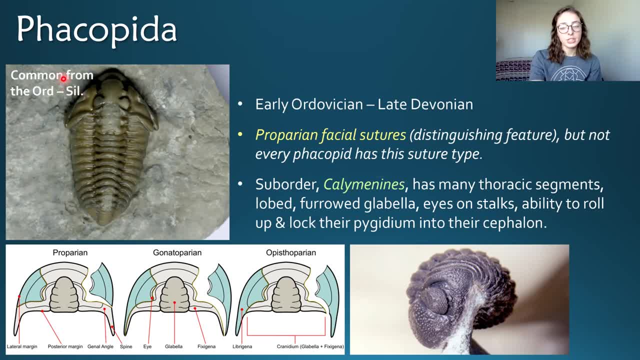 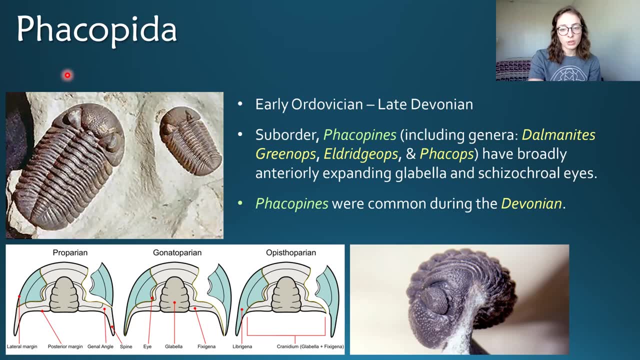 position. Also, these guys were common from the Ordovician to Silurian and, like I mentioned, they have proparion facial sutures that cut off in front of that general angle. The next important sub-order for Phacopids that we'll talk about is the Phacopines, or Phacopines, whatever you want. 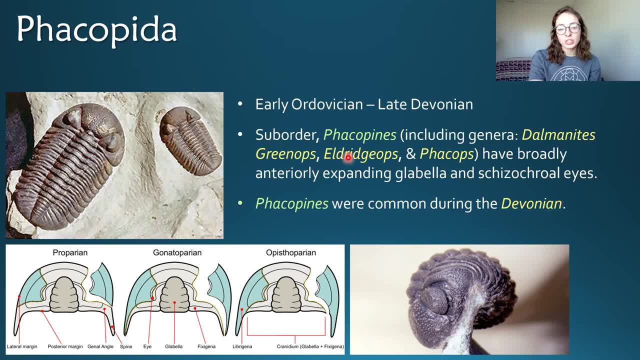 to call it, But these were common in the Devonian and these included some important generalistic as you can see here: Thalamites, Greenops, Eldrigeops and Phacops And these all have broadly anteriorly expanding glabella Shown here in this figure to the left as you can see. 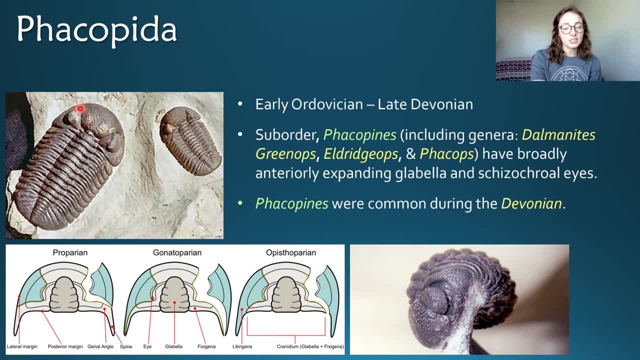 this glabella is huge and it extends toward the anterior or widens toward the anterior of the cephalon. Additionally, they had distinctive schizochral eyes on stalks, as we can see here in more detail at the bottom right picture With all those little dots. those are the lenses. 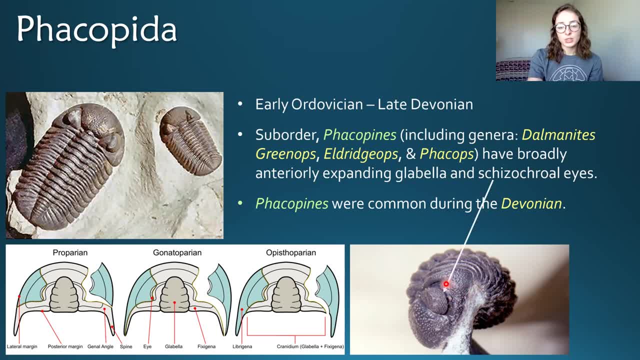 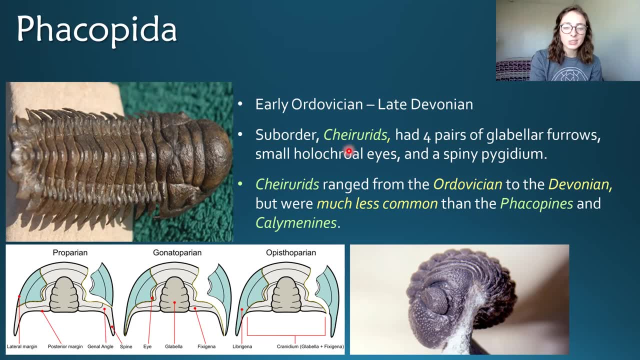 separated by little cuticles in between, And these were distinctive for the Phacopines group. The last sub-order I want to talk about for the Phacopids is the- I should really practice these words before I get into this- Cherurids, I'm going to go with that. So these had four pairs. 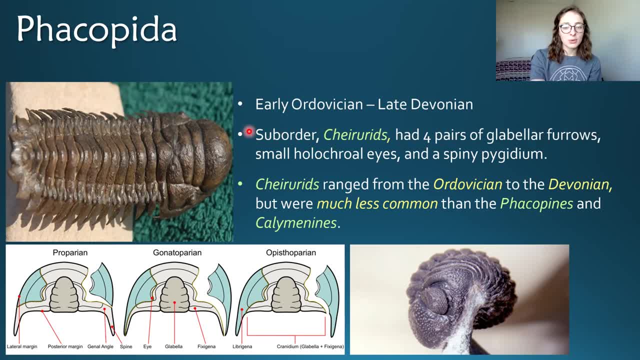 of glabellar furrows, which is really really distinctive for the sub-order. As we can see in this figure, you've got glabellar furrow, glabellar furrow, glabellar furrow and then curved glabellar. 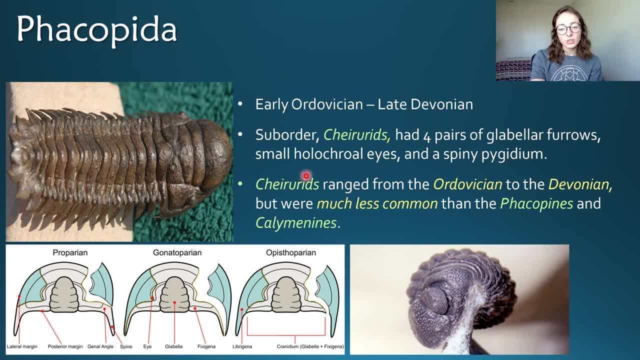 furrow right before the occipital ring And they also have, as you can see, the phallic, which is the phallic eye. They also had small holochral eyes, as we can see protruding from the cephalon. 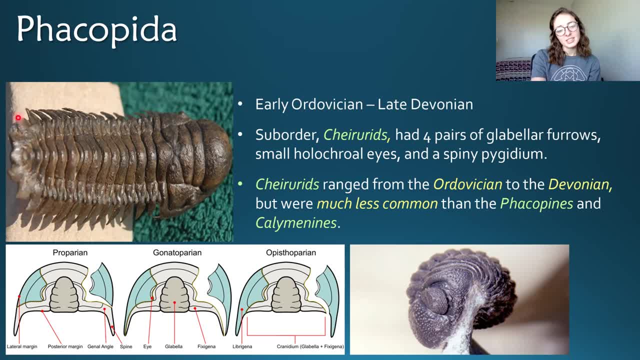 in this figure And they had a spiny pagidium, As we can kind of see at the back of this guy. they had some little spines back here Also. they ranged from the Ordovician to Devonian, but were much less common than the Phacopines and Calamonines sub-orders. 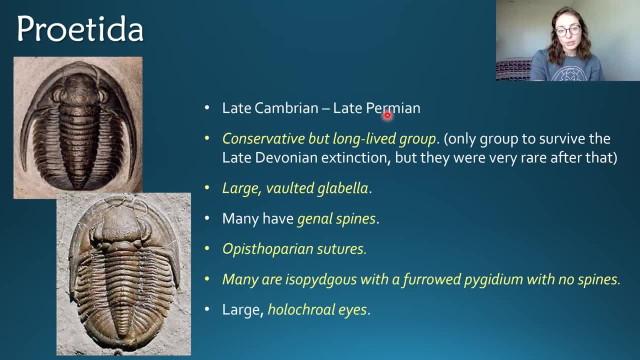 Next we have the Proedids which went from the Late Cambrian to Late Permian And, as we can see, this is the only group so far we've talked about that has survived to the Permian And actually, as we'll see later when we talk about trilobite evolution, these are the only. 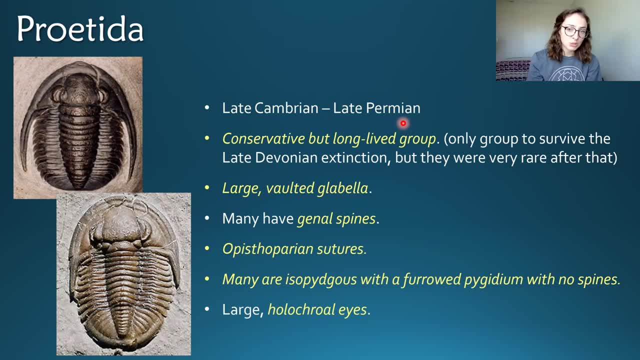 Ordo trilobites that survived to the Permian because they were able to survive both the Ordovician and Devonian extinctions, unlike the other trilobites. Additionally, they had a large vaulted glabella, as we can see here in these pictures. Also, they have long gentle spines. 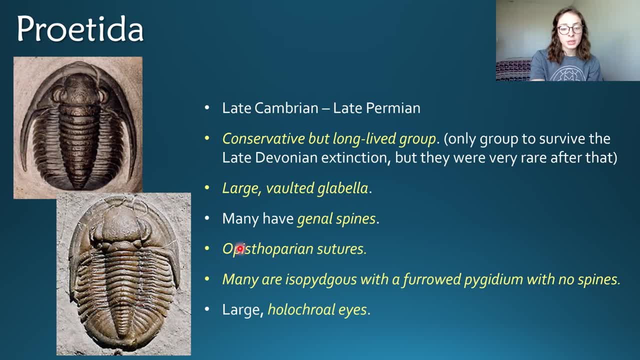 as we can see in these groups and these pictures, And they have opisthoperian sutures, like many other groups of trilobites we've talked about, And many are isopygous, a Pagidium similar in size to their Cephalon, and have a furrowed Pagidium with no spines. So 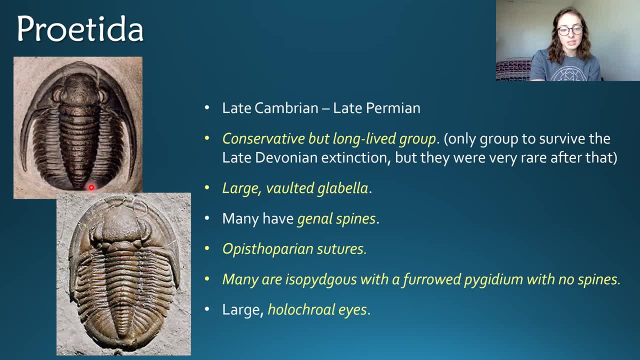 we can see. it's pretty distinctive that these two pictures here. there are no spines on the Pagidium And that's a distinctive feature of these Proedids. Also, they have large holochral eyes. You can see the large crescent shapes here on either side of their glabella. These 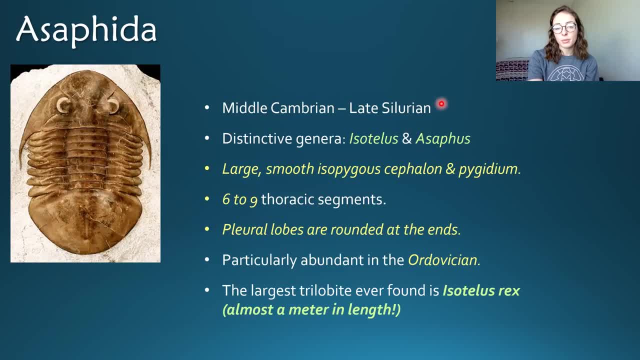 are their large holochral eyes. Next we have the Asaphids, which went from the Middle Cambrian to Late Silurian, which have distinctive genera, including Isotelus and Asaphis, which will show up on the next slide when we talk about the size of these guys, because these guys got pretty big. 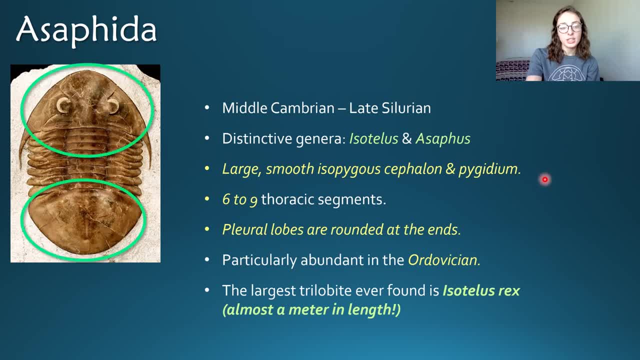 Also they have a large, smooth, isopygous Cephalon and Pagidium, as shown in this picture. Also, they have six to nine thoracic segments, which, if you feel like counting the thoracic segments, could be a distinctive feature. Also, they have pleural lobes that are rounded at the end. So 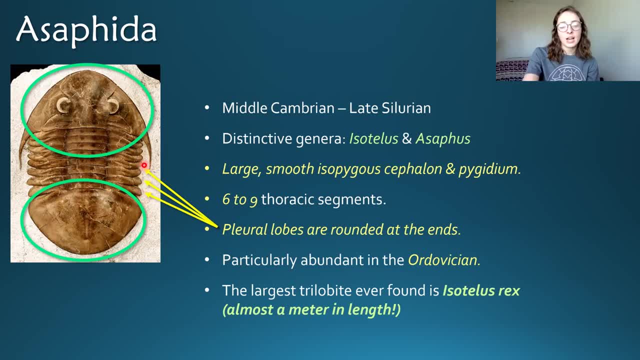 we can see, they're not like spiny, They're more rounded. That's a distinctive feature of these guys. Also, they are particularly abundant in the Ordovician and they include the largest trilobite that ever lived, And that is the Isotelus. 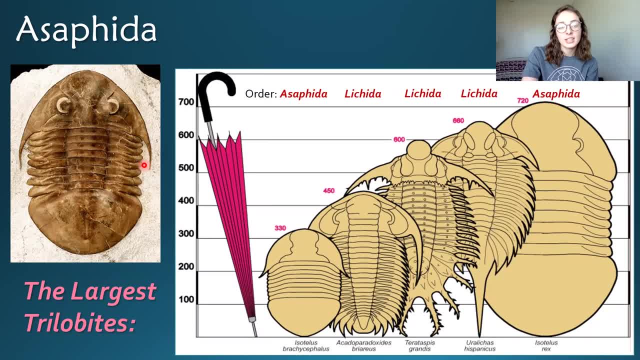 Isotelus rex, which got to almost a meter in length. Here is an image showing the largest trilobites to ever have lived. This includes one species of Isotelus at the lower end of the larger trilobite sizes, And this is still pretty big, at around 300 millimeters Then. 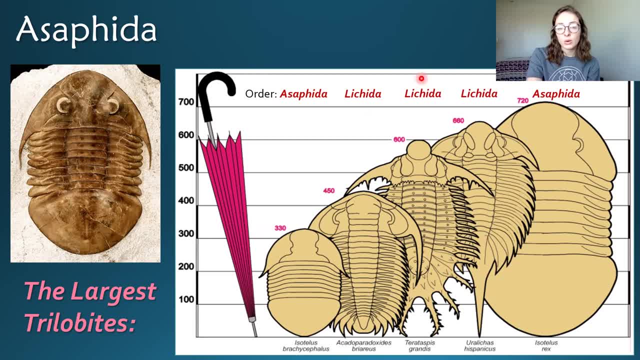 you have three genera shown here in the middle that are actually part of the Lichida order, And these genera also got very big, anywhere from 450 to almost 700 millimeters. Then you have the Isotelus rex, which is one of the Asaphids we just talked about. 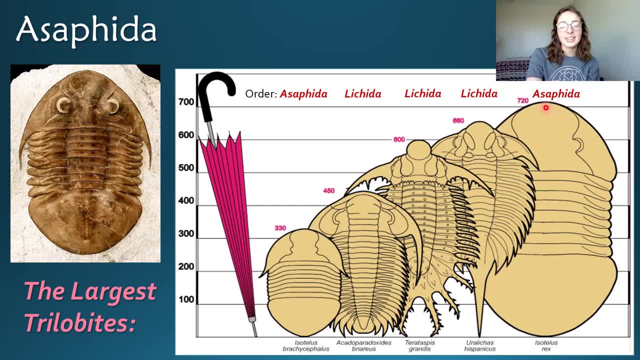 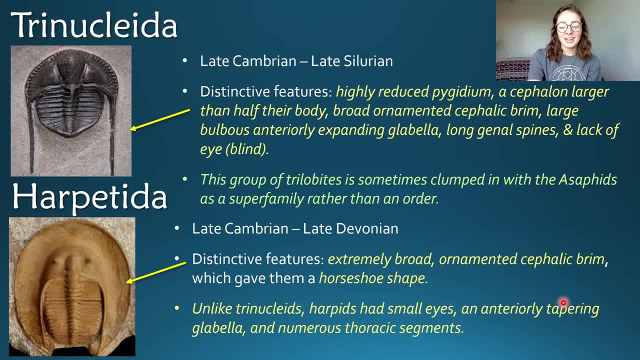 that got to around 720 millimeters in length. Next we have the Trinucleids and Harpida. That actually says Harpatida, but that's supposed to say Harpida, by the way. But basically the Trinucleids went from the Cambrian to late Silurian And their distinctive features include: 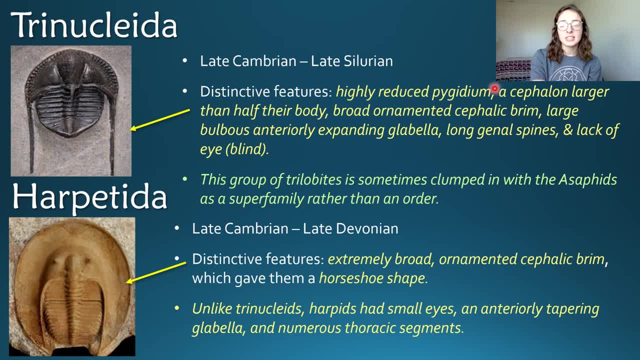 a highly reduced Pugidium. so tiny Pugidium down here, A Cephalon larger than half their body typically. So we can see here they have a huge Cephalon compared to their little body And they. 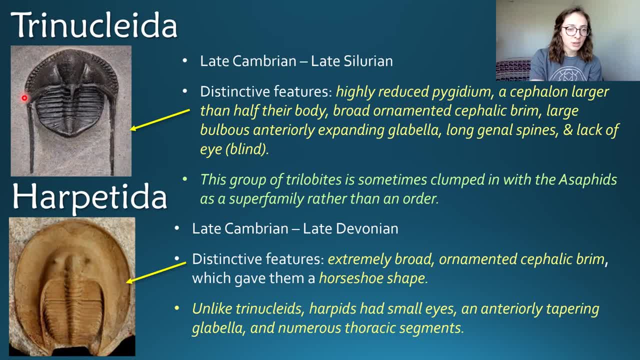 have broad ornamented cephalic brims So we can see their cephalic brims here Kind of looks ornamented in a way, And that's typical of Trinucleids. They also have a large bulbous anteriorly expanding glabella as shown here. It's expanding toward the anterior. 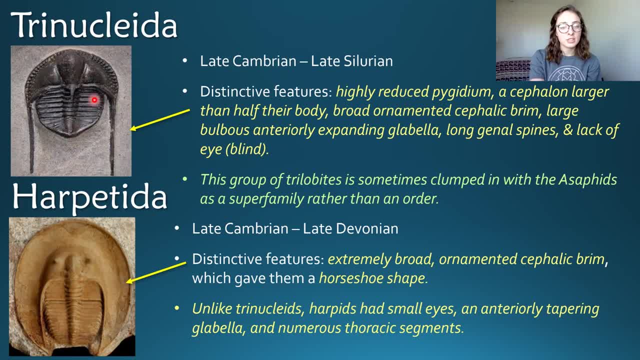 and it's pretty bulbous and large And they have long gentle spines, as shown here- Pretty distinctive but may not be preserved, And they have a lack of eyes. aka, they were blind. Also a disclaimer: this group of Trilobites is sometimes clumped in with the Asaphids. 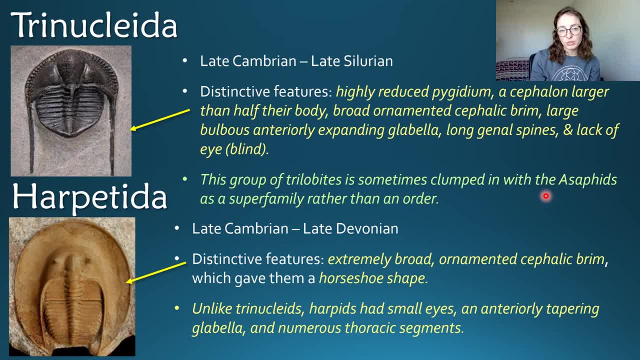 as a superfamily rather than its own order, And so sometimes, if you read about Trilobite orders, they may not include Trinucleids as one of them, because they clump it in with the Asaphids. 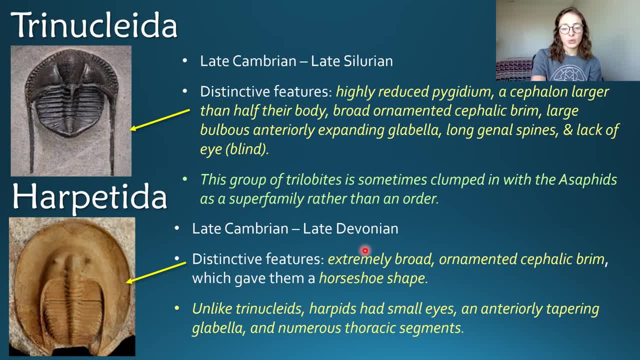 Also, we have the Harpids, which went from the late Cambrian to late Devonian, And they have distinctive features, including extremely broad ornamented cephalic brim Which, as you can see here in this case isn't super ornamented but is extremely broad, much more broad. 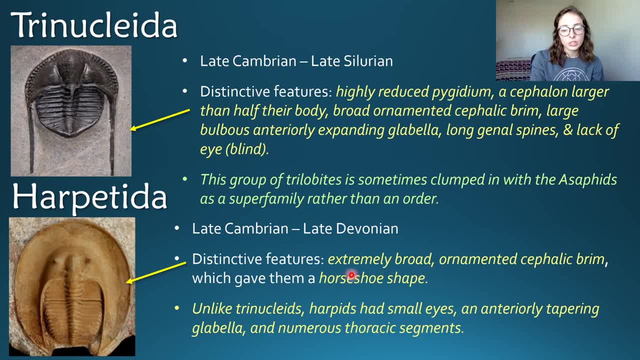 than the brim of the Trinucleid here, And they have a distinctive horseshoe shape because of this, Because their cephalic brim is so broad and goes down so far that it looks like they are basically like a horseshoe crab. And, unlike Trinucleids, Harpids had small eyes, so they 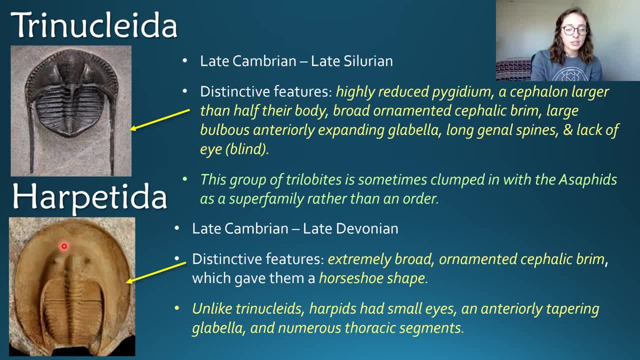 weren't blind And they had interiorly tapering glabella rather than expanding glabella. So their glabella is narrowing toward the anterior of their cephalic brim rather than expanding or widening. And they had numerous thoracic segments compared to the Trinucleids, which 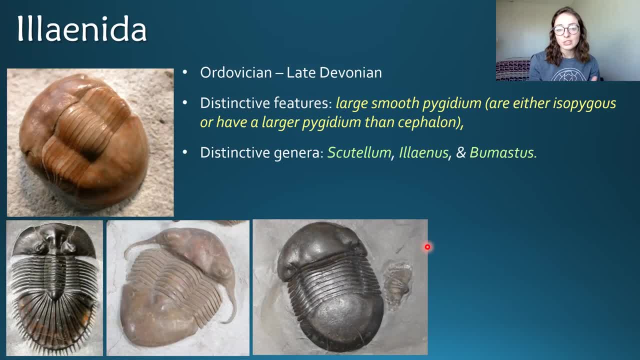 did not. So now we can move on to the last order of Trilobites, which is the Elanids. This group of Trilobites went from the Ordovician to late Devonian And they have distinctive features. 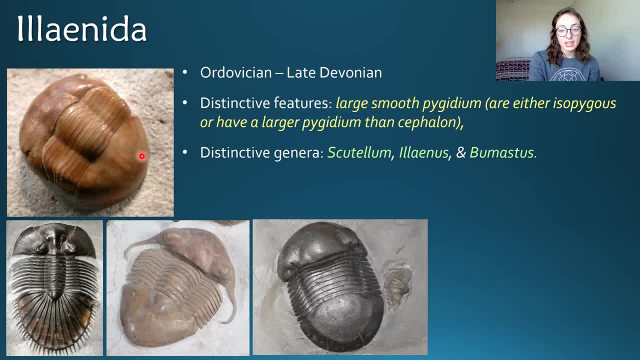 including a large, smooth Paginium, which we can see here, is smooth and has hardly any ornamentation or segmentation or anything, And so that's a typical feature, As well as sometimes being isopygous or even having a larger Paginium than their Cephalon And distinctive genera of this. 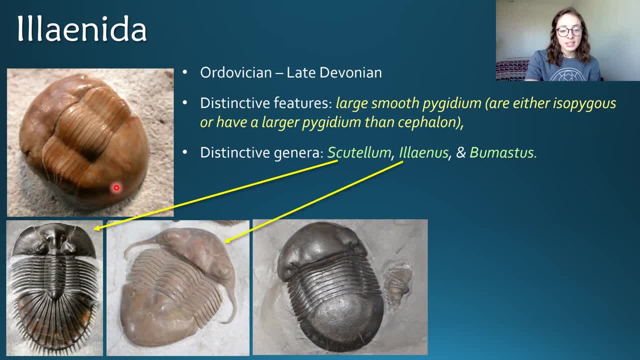 order include Scotellum, shown here to the bottom left, Elanids, shown here in the middle, with these interesting little gentle spines here that curve in, And then Bumastis, which is my favorite because I remember it by thinking of its little bum. 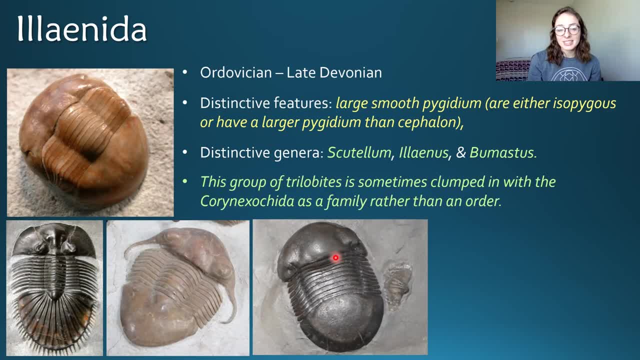 It's near equal in size or even bigger than its Cephalon. But there's a disclaimer here as well: This group of Trilobites is actually often clumped in with the Corynexicids as a family rather than. 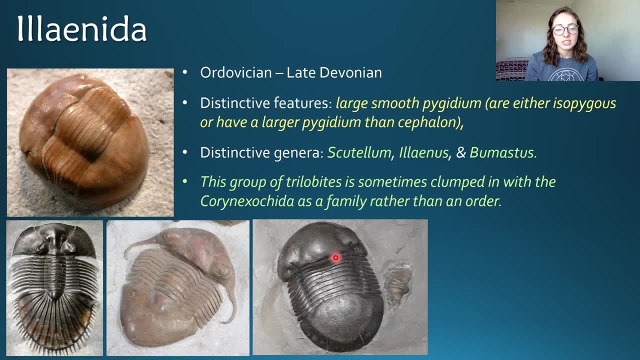 its own order, similar to the Trinucleids. So sometimes if you see a list of Trilobite orders and the Elanids aren't on there, it's because they're thought to be within the Corynexicids. 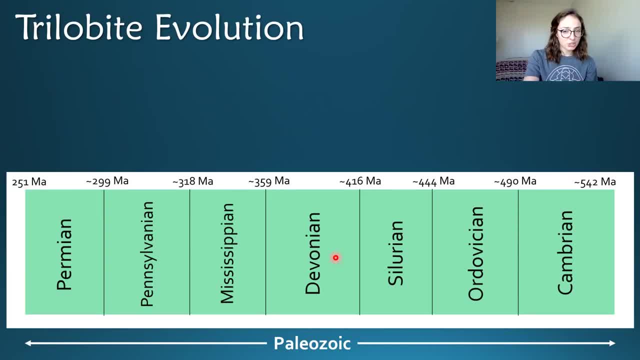 Now we can get to Trilobite evolution. We'll talk about their general evolution on this slide and then their more specific order by order evolution on the next slide. So on this slide we can see that the Promo-Triassic extinction started in the late Cambrian. They reached their 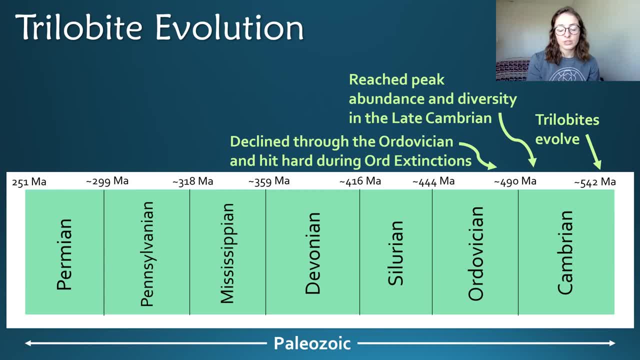 peak abundance and diversity in the late Cambrian. They declined through the Ordovician and were hit hard during the Ordovician extinctions. But many survived to the late Devonian, only to be hit hard again by the Devonian extinctions. And then, like we mentioned earlier, only one order survived until. 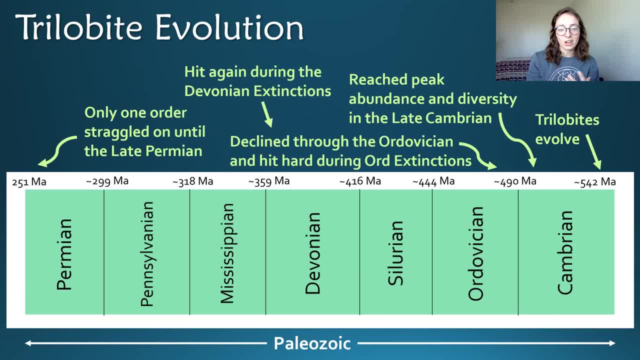 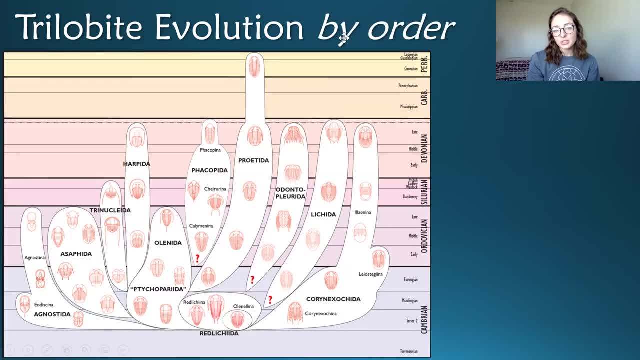 the late Permian, That was the Proedids, And they weren't super abundant either. They kind of just straggled on past the late Devonian into the late Permian until they finally went extinct at the Promo-Triassic extinction. So now, getting to the Ordovician, and I'm going to show you a couple of